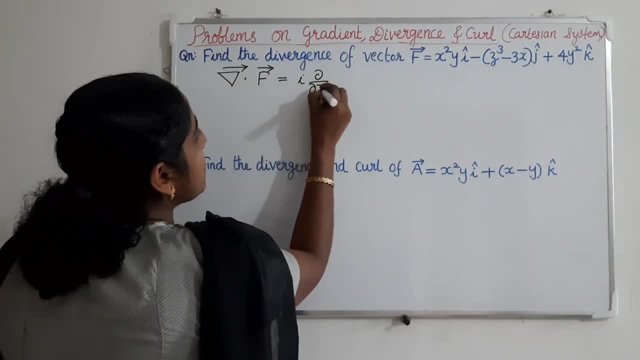 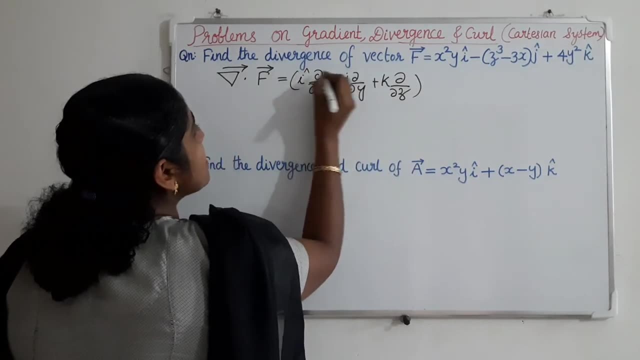 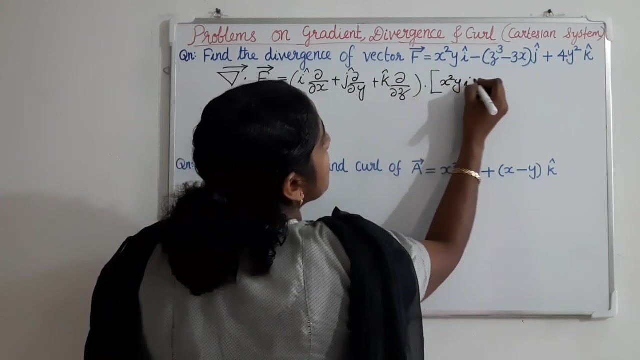 What is it? This is del operator i. dou by dou x plus j. dou by dou y plus k, dou by dou z, where i, j, k are unit vectors along x, y, z axis. Dot f vector, that is x square y i minus z. cube minus 3x j. 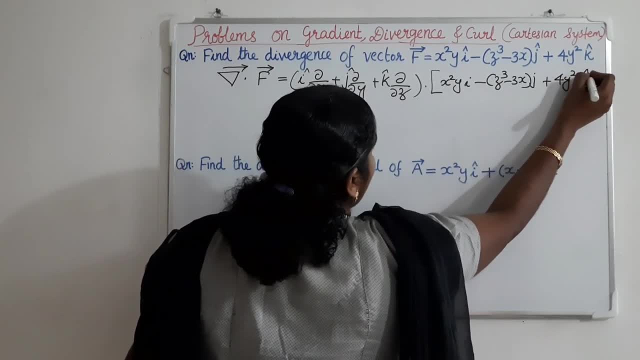 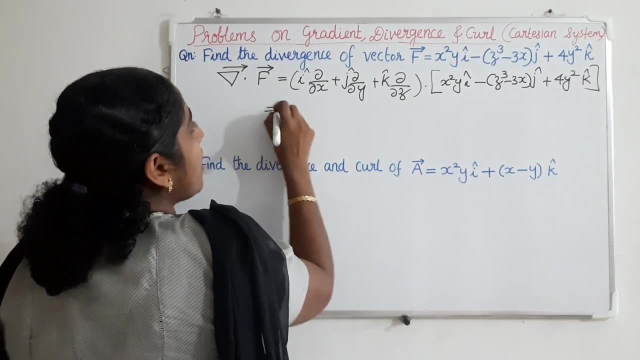 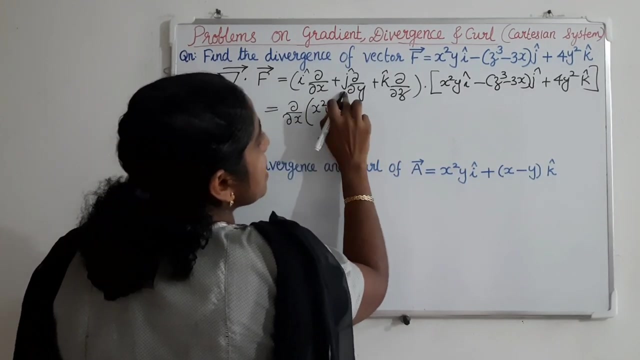 plus 4y square k. So while taking the dot product, only i dot i, j dot, j, k, dot k will come, so all other terms become 0.. That is i dot i. that is when the coefficient is dou by dou x of x square y plus j and j. 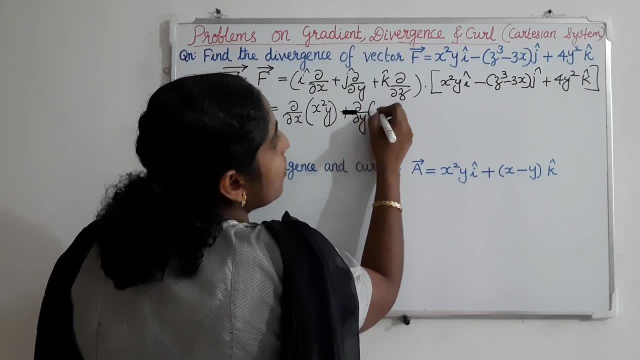 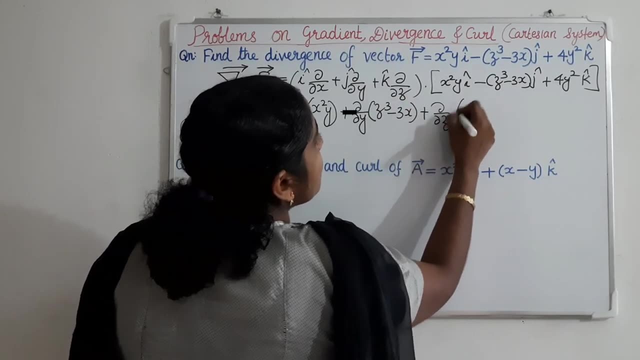 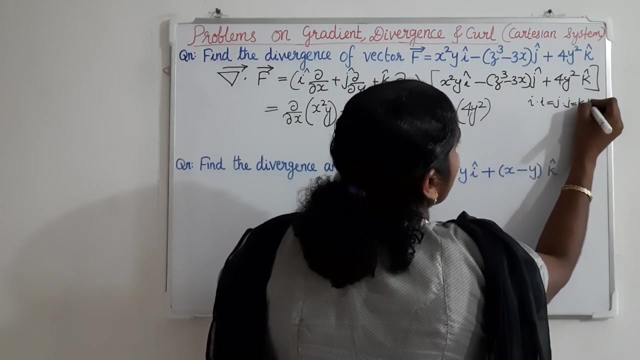 components here are: dou by dou y of z cube minus 3x, plus dou by dou z of 4y square, because i dot i is equal to j, dot j is equal to k, dot k is equal to 1 and i dot j is equal to j, dot k is equal to 1.. 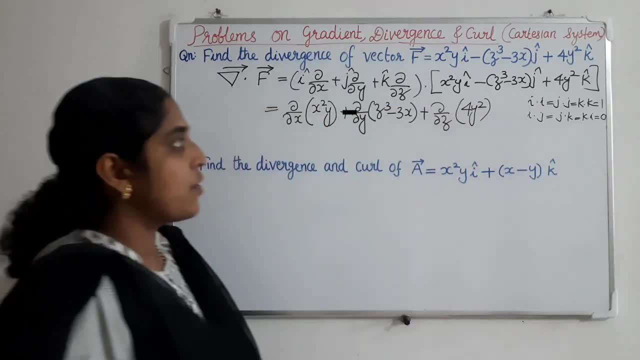 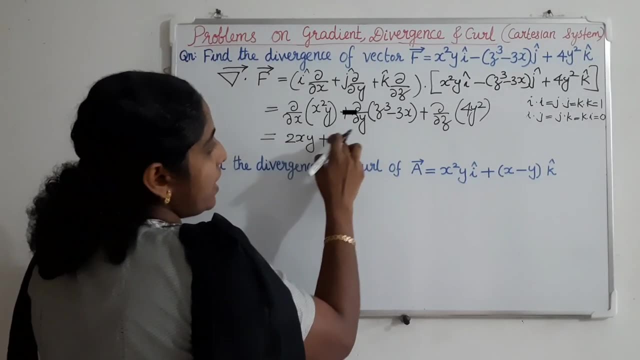 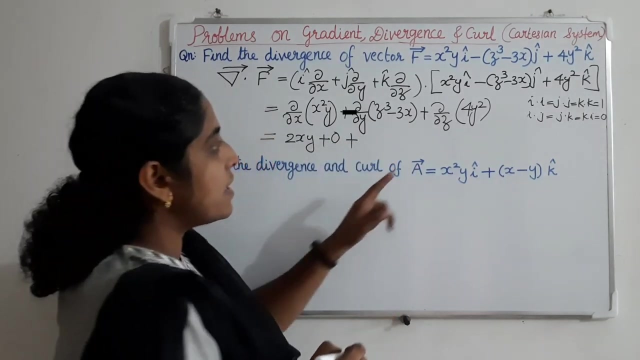 So here this dou by dou x of x square y is 2xy plus dou by dou y, that is partial derivative of z cube minus 3x with respect to y, is 0 plus dou by dou z of 4y square. there is no z components, since it is partial derivative. here also the answer is 0.. 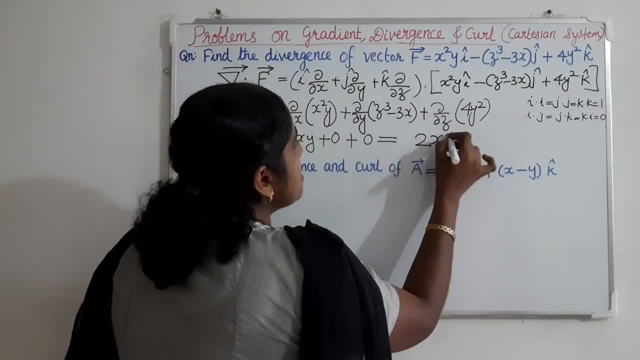 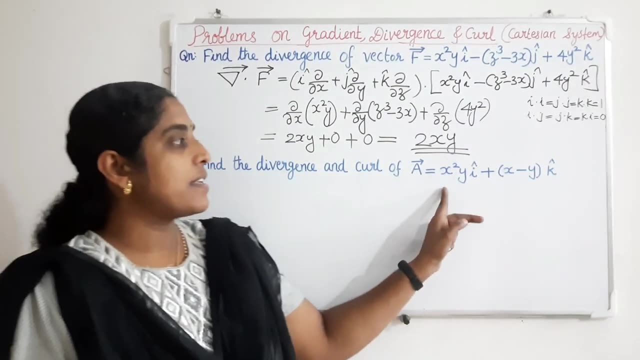 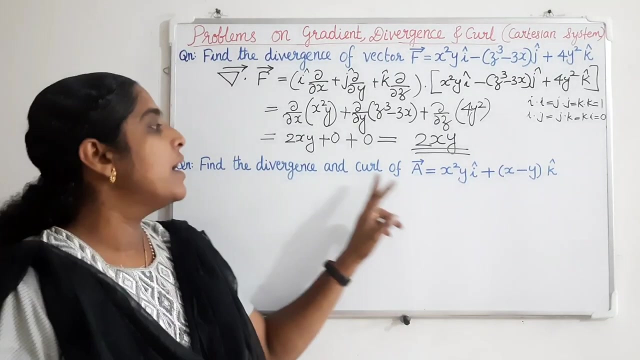 So far it will be del dot f. del dot f is 2xy. Now find the divergence and curl of a vector is equal to x square y i plus x minus y, k. Here this divergence means del dot a vector, curl means del cross a vector. 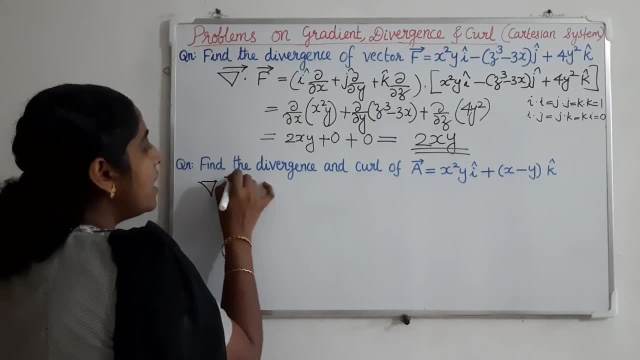 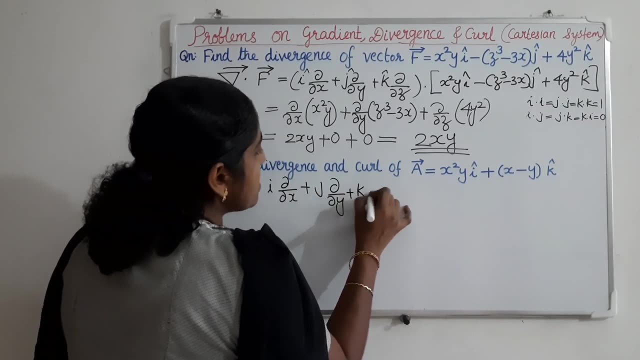 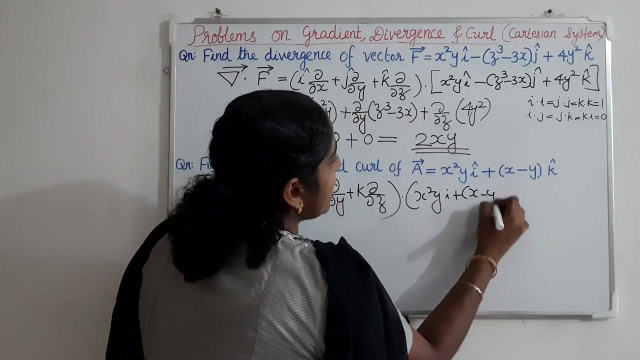 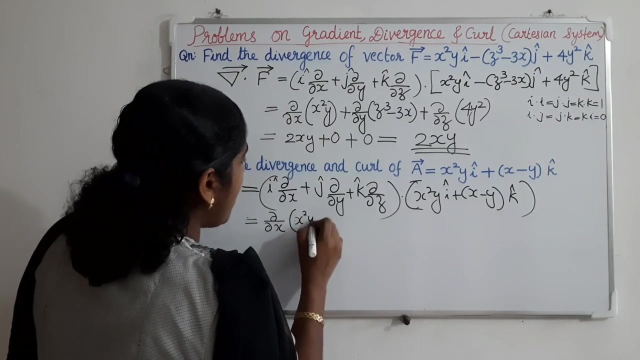 So first we can find out the divergence, that is del dot a vector. So del is i. dou by dou x plus j. dou by dou y plus k. dou by dou z. dot a vector is x square y i plus x minus y k. That is dou by dou x. of the i and i components are x square y plus here j component is dou. 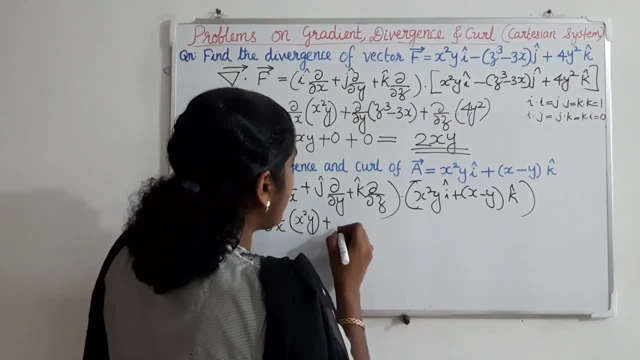 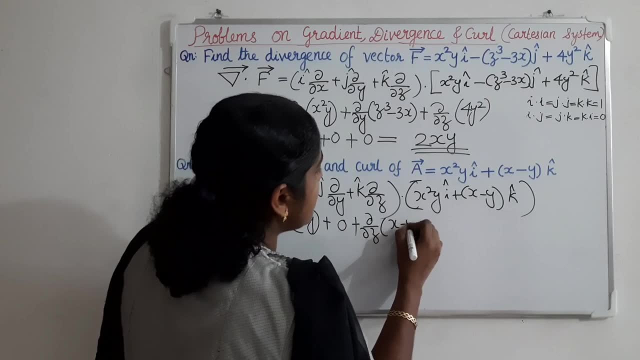 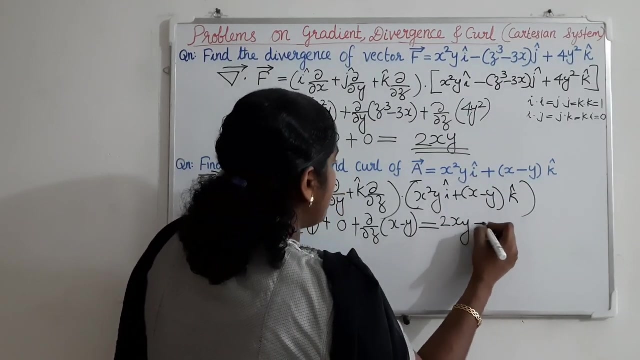 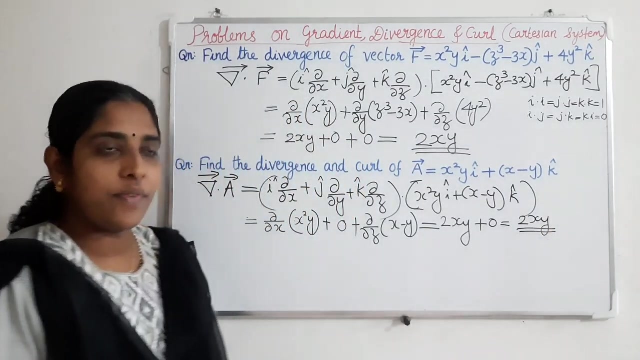 by dou y, but in vector there is no j component, so that is 0 plus k component. yeah, dou by dou z of x minus y, that is equal to dou by dou x of x. square y is 2xy plus dou by dou z of x minus y is 0. So the divergence of the given vector is 2xy. Now we have to find out. 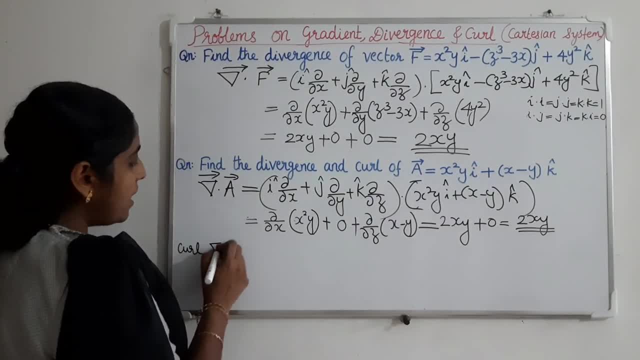 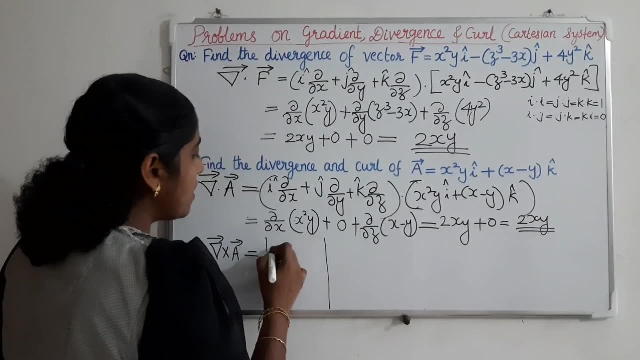 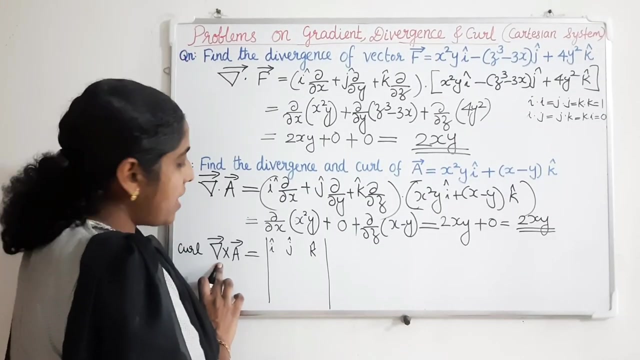 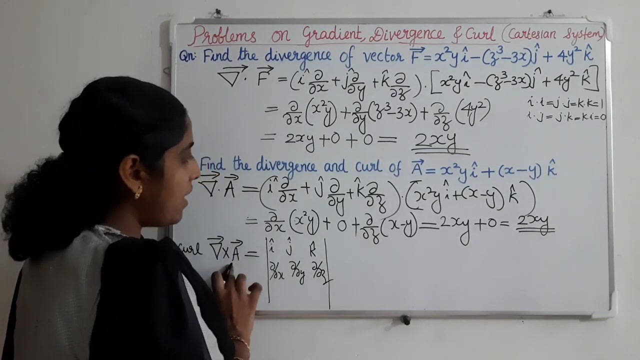 the curl of A. So what is curl? Curl means del cross A vector. How to find out the curl of a vector? For that we can use the determinant method. The first row is i, j, k. Second row is components of del along i j k axis, that is, dou by dou x, dou by dou y, dou by dou z and A. 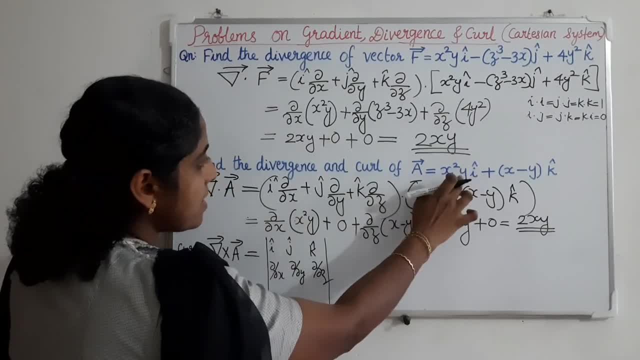 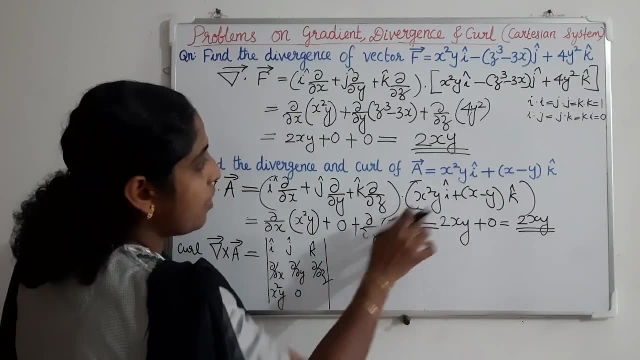 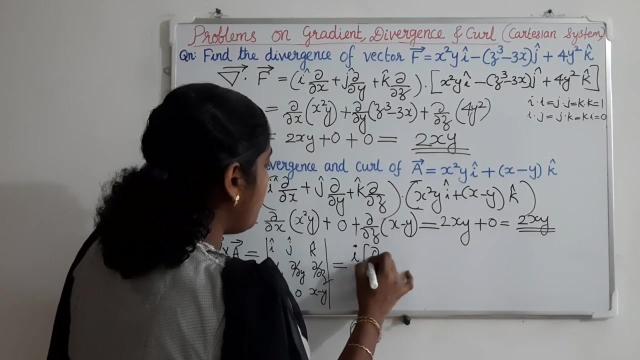 vector components along x, y, z axis are this: x component is x square y y component. there is no y component, So here it is 0.. Z component is x minus y. So using the determinant method, i into dou by dou, y of x. 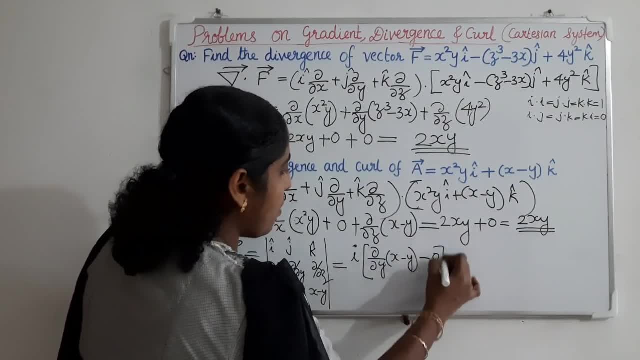 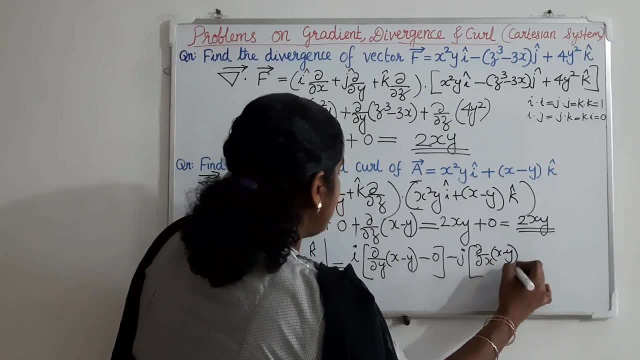 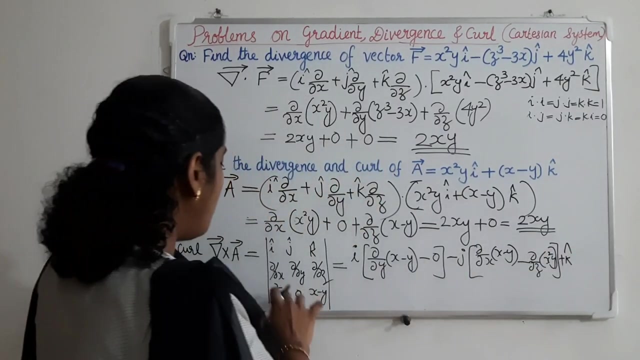 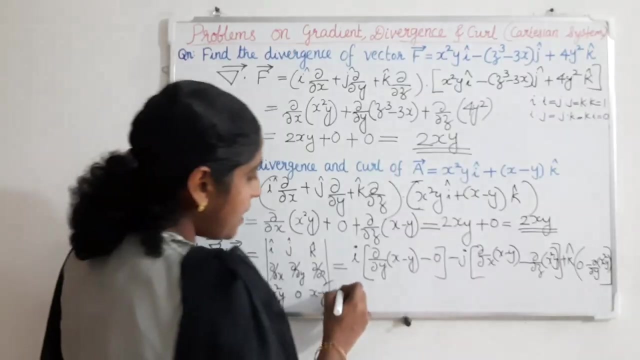 minus y minus dou by dou z of 0 is 0 minus j. into dou by dou x of x minus y minus dou by dou z of x square y plus k. into dou by dou x of 0 minus dou by dou y of x square y, That is equal to i. 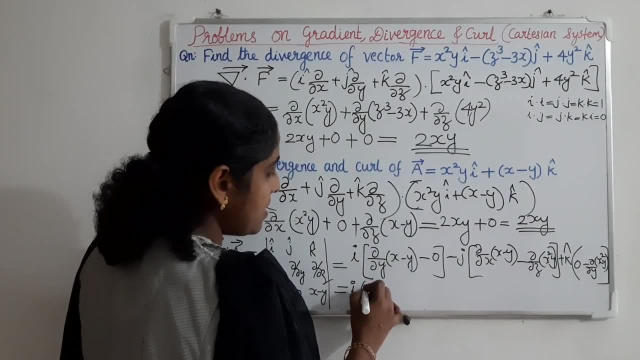 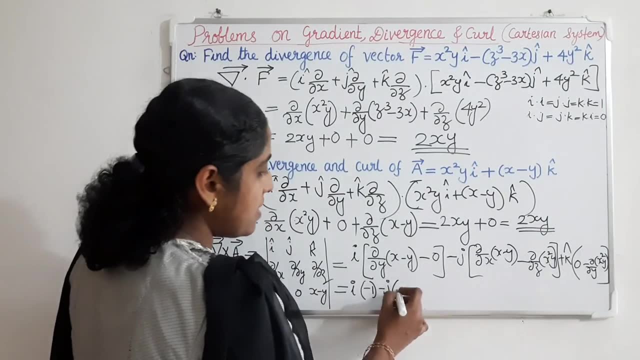 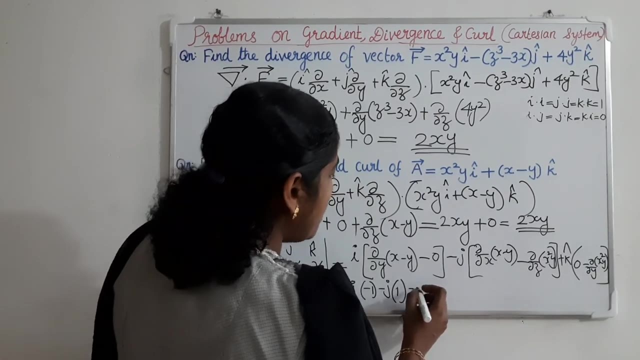 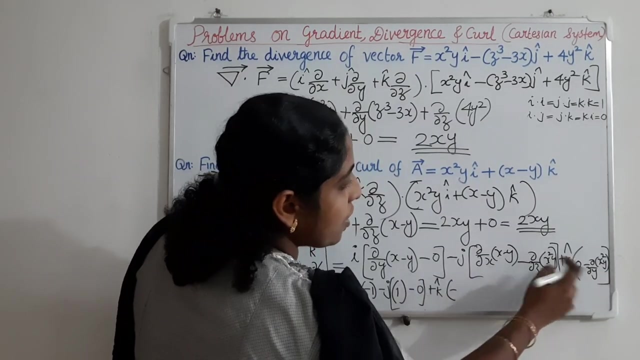 into dou by dou y of x minus y, that is minus 1 minus j. into dou by dou x of x minus y, that is 1 minus dou. by dou z of x square y, that is 0 because there is no z components there- plus k. into minus of dou by dou y of x square y. 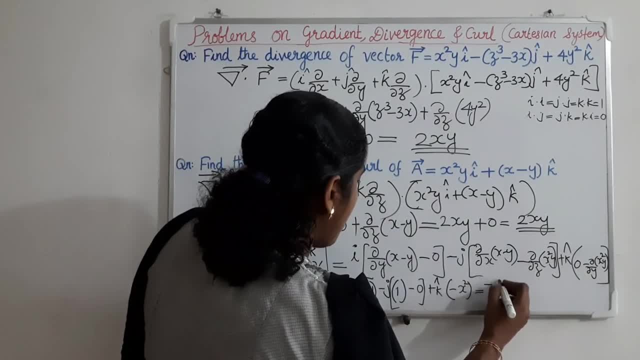 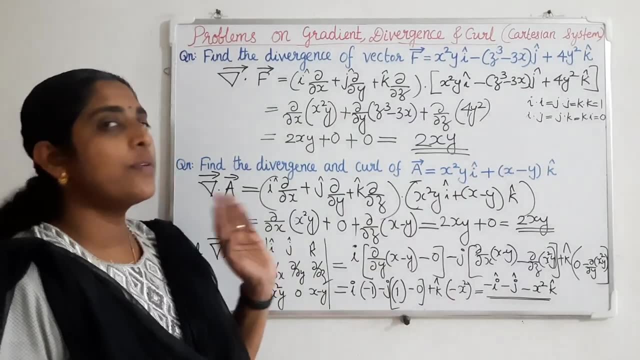 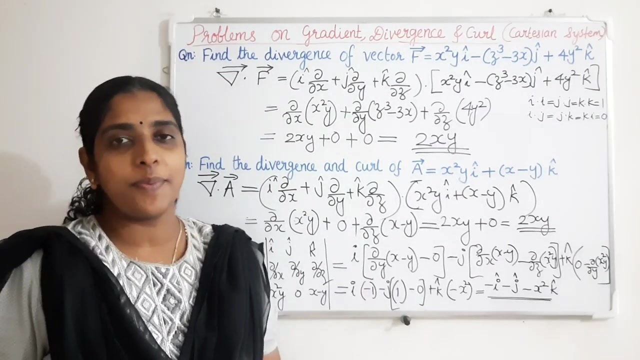 that is x square. that is equal to minus i minus j, minus x square k. So this is the curl of the given vector. So divergence of a vector we can find out by taking the dot product and curl of the vector we can find out using the cross product. See the next question. If your scalar field phi, 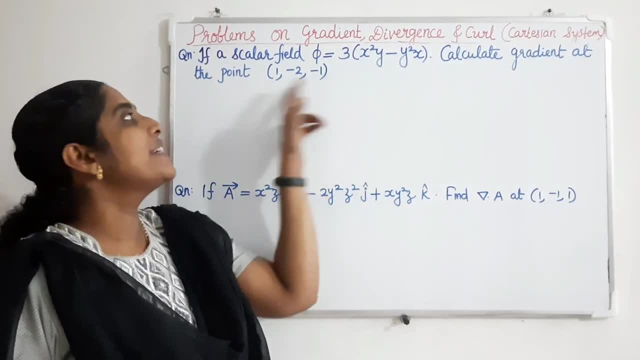 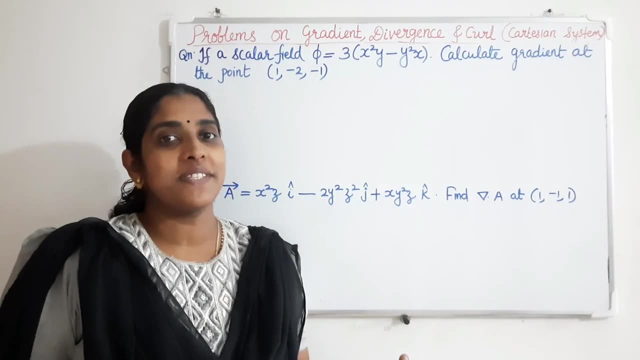 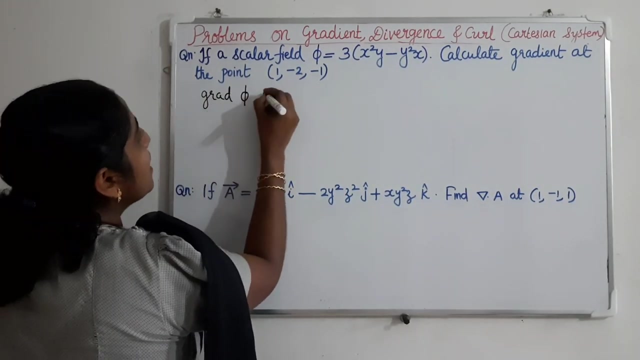 equal to 3 into x square y minus y square x. Calculate the gradient at the point 1 minus 2 minus 1.. What is gradient? That is, when del operates on the scalar function, what we are getting is gradient. So to find out the gradient of this scalar function, we can take the del operator on this. 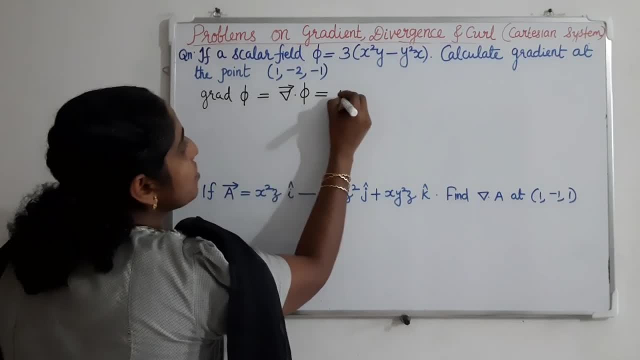 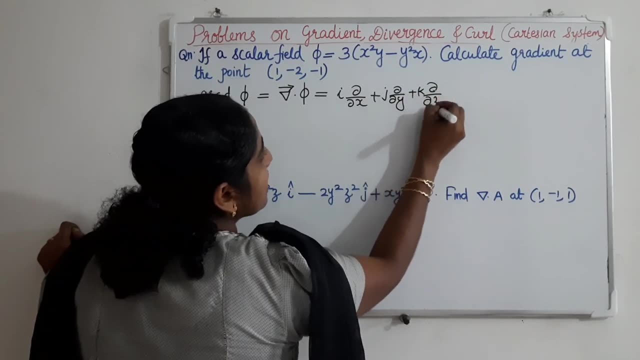 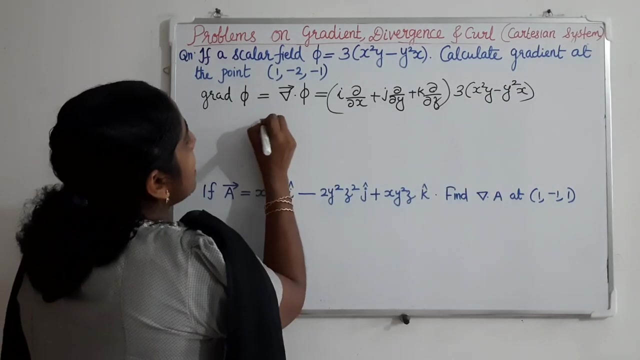 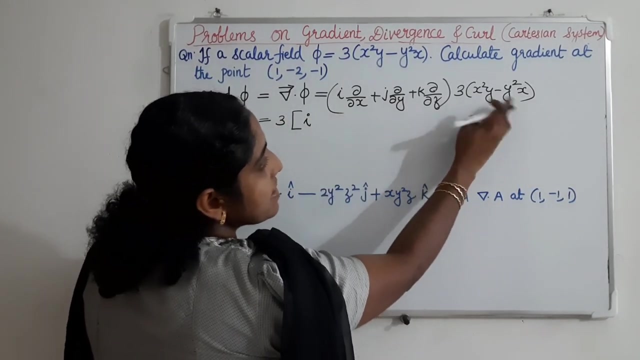 function that is del phi. So that is equal to i dou by dou x plus j. dou by dou y plus k. dou by dou z, which is acting on the function 3 into x square y minus y square x. That is, 3 is the constant that we can take outside I into dou by dou x of x square y minus. 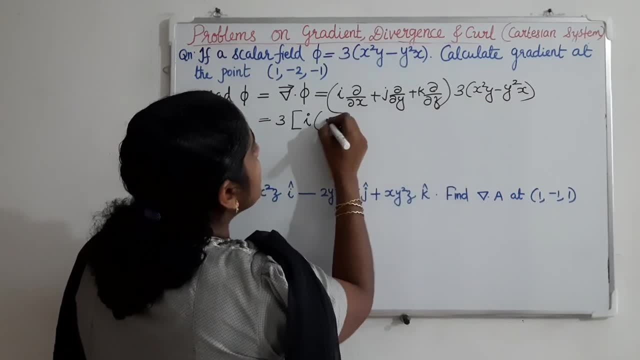 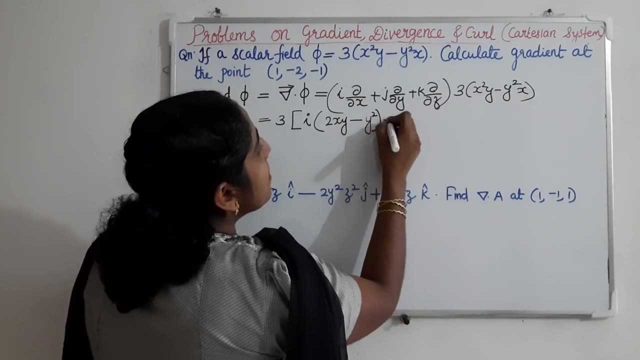 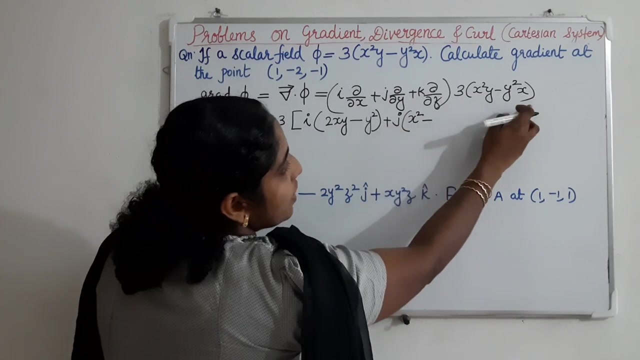 y square x. So when it is acting on x square y, this is 2xy minus. the partial derivative of y square x is y square plus j into dou by dou y of this x square y, that is x square minus y square x is 2y x plus k into dou by dou y of x square y, that is 3 into dou by dou x plus j into dou y of x. 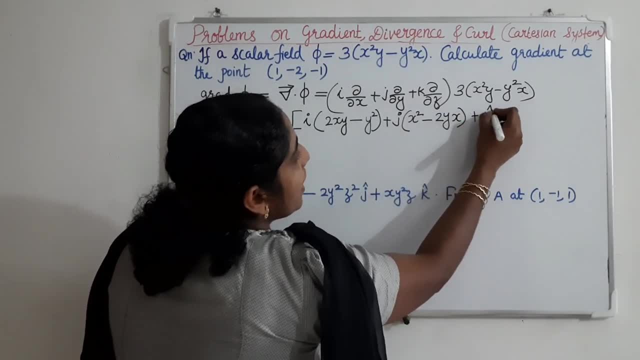 square y minus y square. If there is no del externally related multiplication, then we have a error. in® vector of k divided by So waveız is far spires. that is a straight lineści at a high diagonal. so there arebstudet to it better. 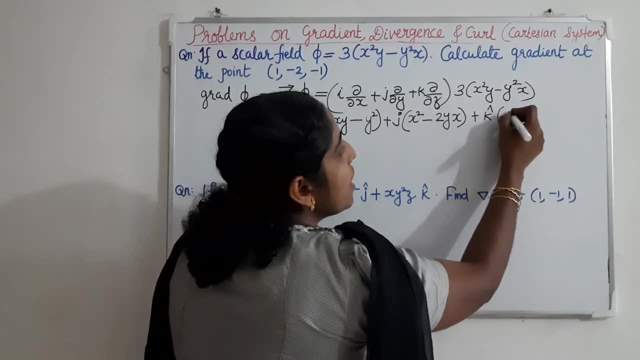 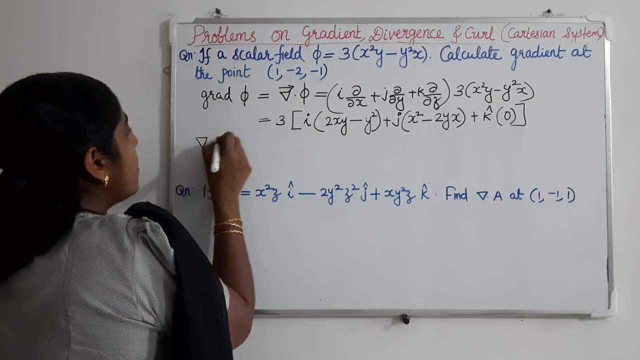 be a straight lineell og, assuming also the derivative with fact there is also space in-referential or for any other dou z. there is no z component over this function, so k component is 0. now we have to calculate this gradient at the given point. that is what is del phi at the point 1 minus 2 minus 1 for that: 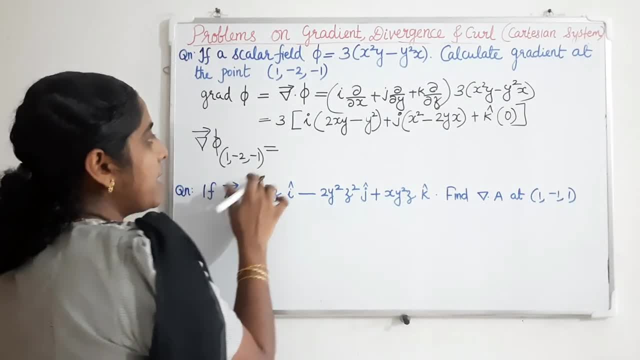 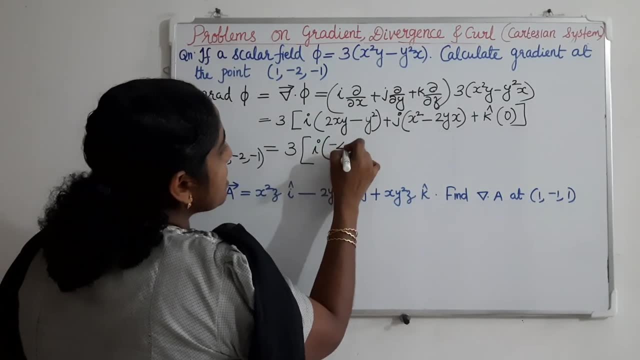 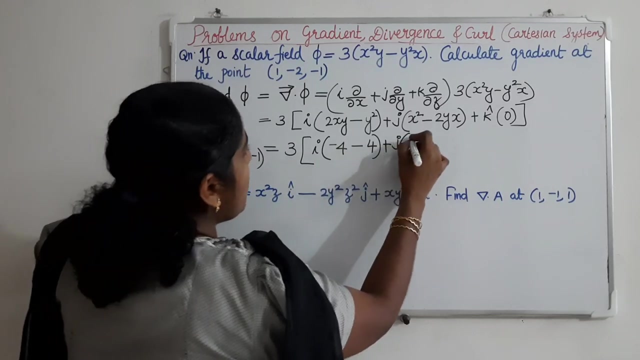 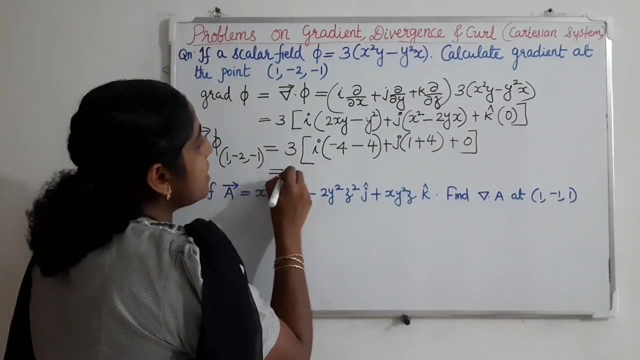 substitute x as 1, y minus 2, z as minus 1. so 3 into i, into 2, into x: y is minus 2, that is minus 4 minus y. square is 4 plus j. into x. square is 1 minus 2 y, x. that is so plus 4 plus 0, that is. 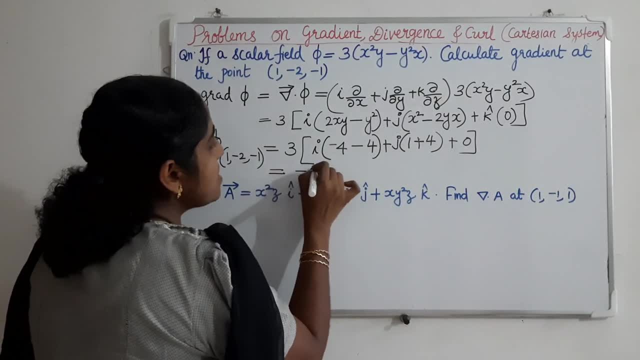 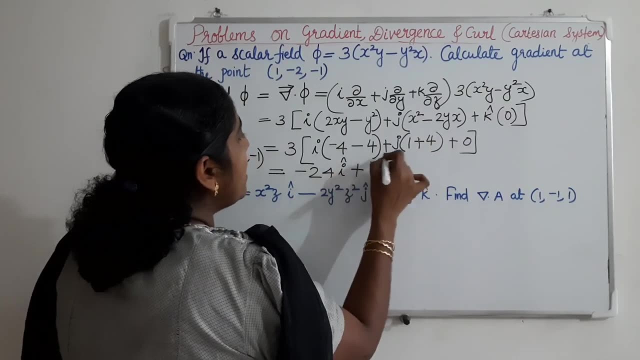 minus 4 minus 4 minus 8 minus 8 into 3 is minus 24. i plus 4 plus 1, 5 into 3, 15 j. so this is the gradient of the function at the given point. gradient of a scalar function is a. 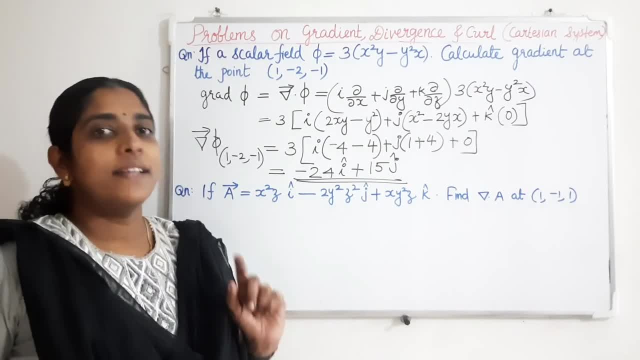 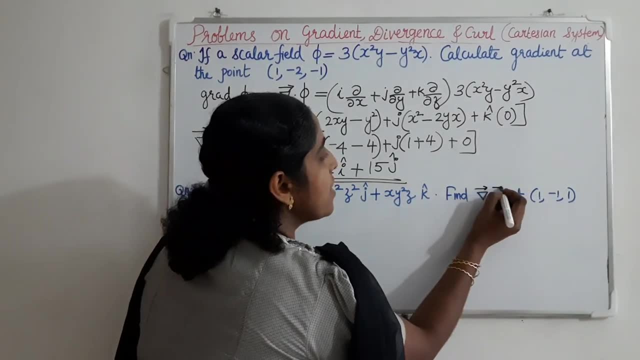 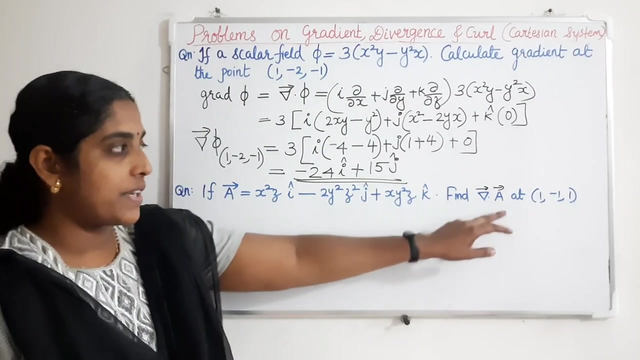 vector, that is gradient, is a directional derivative. next question: if a vector equal to this, find del, dot a at a 1 minus 1, 1, so here we have to find out the divergence, because the given function is vector. so when del operate on the vector function by a dot product that is known as the 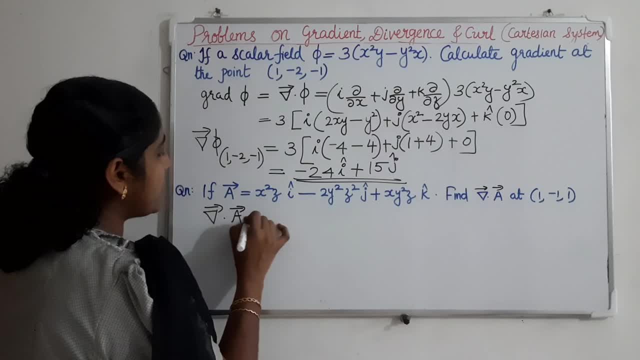 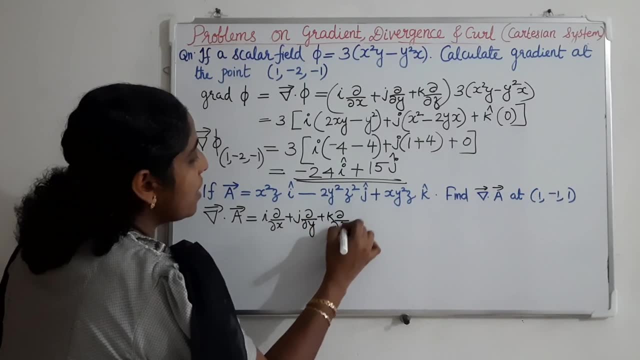 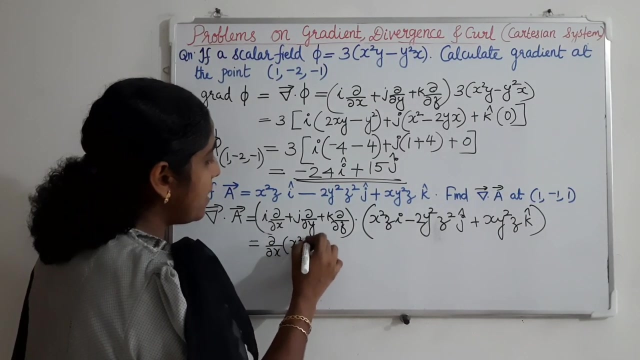 divergence. so what will be divergence of the given vector, that is, i dou by dou x plus j, dou by dou y plus k, dou by dou z dot this function, that is equal to dou by dou x of x square z, plus dou by dou y of minus generally. 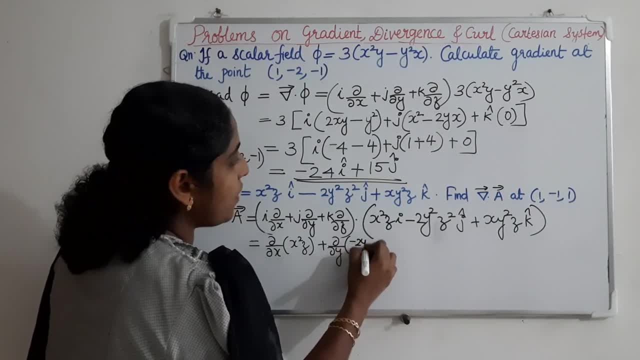 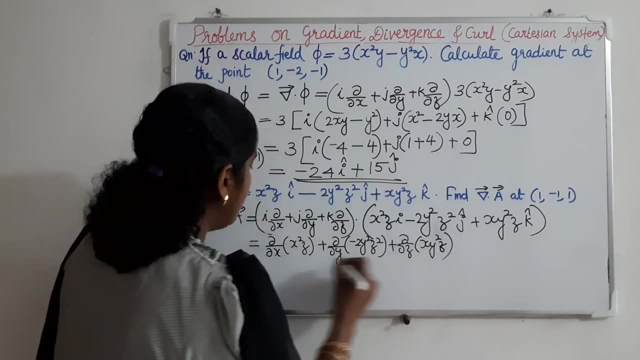 goes 모² minus 2 y square z square plus dou by dou z of x y square z, so it is equal 2 golxz of x- y square z, so it is equal to 2 xz plus minus 4 y z square plus x y. Moreover, 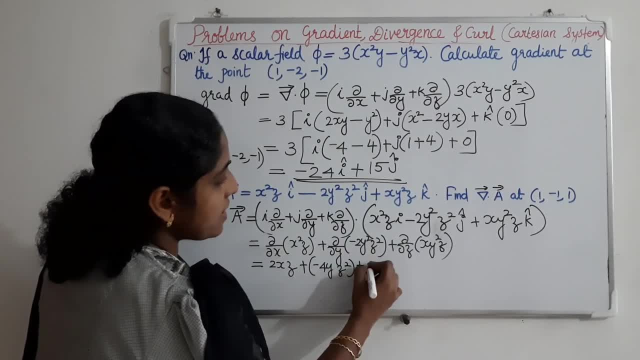 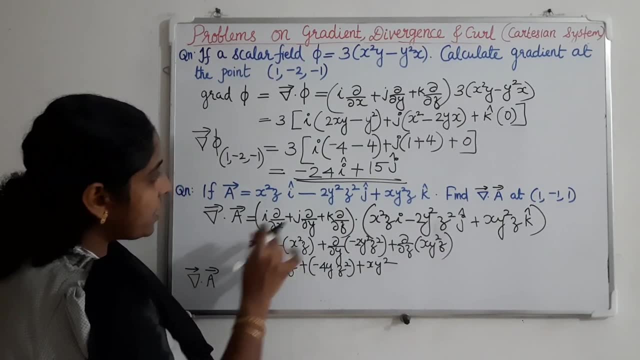 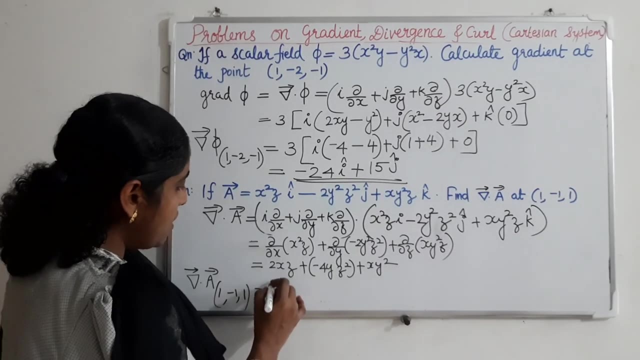 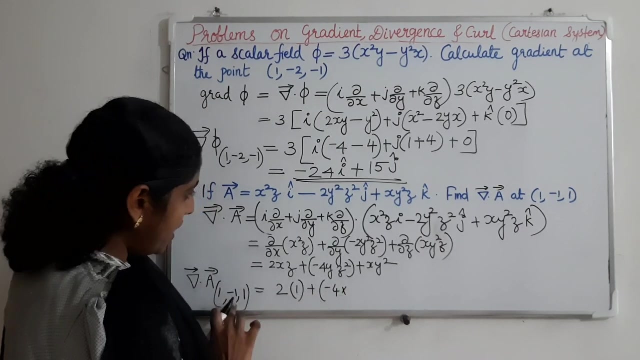 that isgelроб Make filtering very easy. だ ふap square. Now we have to find out the del dot a at what point. that is 1 minus 1, 1.. So we can substitute this xyz in this expression. So we will get 2 into xz, is 1 plus minus 4 into yz square. 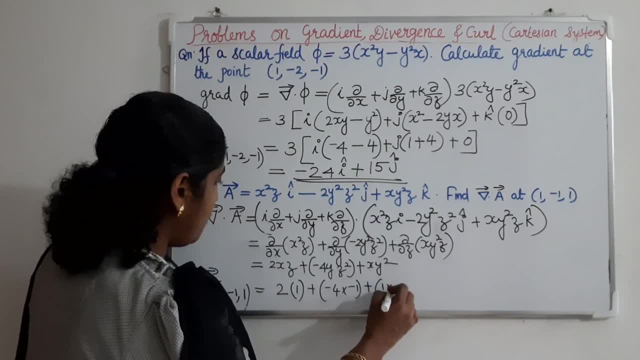 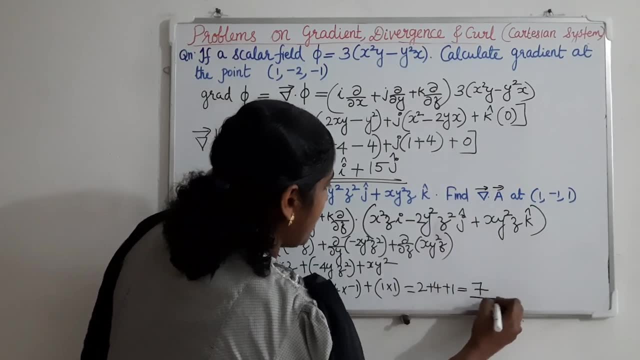 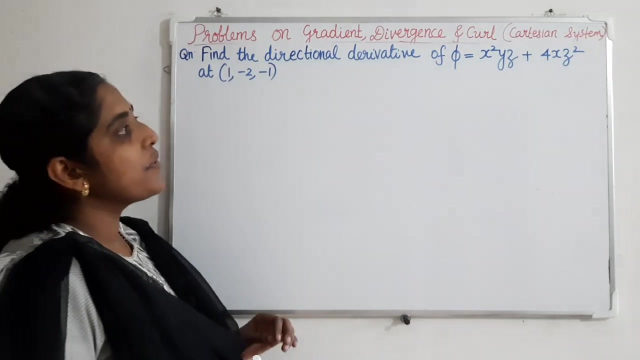 is minus 1 plus x into y square is 1.. That is 2 plus 4 plus 1, that is equal to 7.. So the divergence of this function at the given point is 7.. See the next question. Find the directional derivative of. 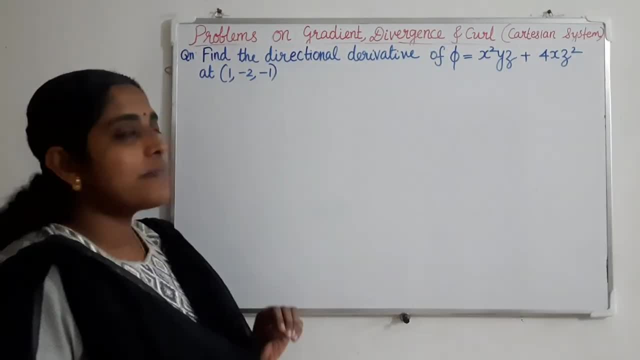 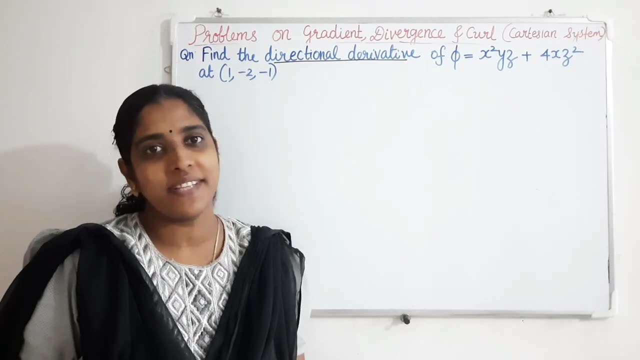 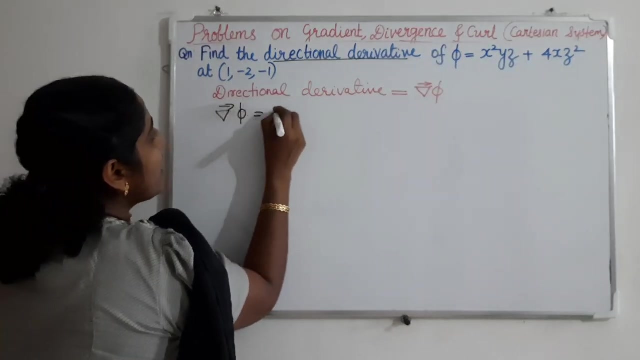 i equal to x square, yz plus 4, xz square at 1 minus 2 minus 1.. What is directional derivative? Directional derivative means gradient of the given scalar function. So in this question we have to find out del phi. So del phi is equal to i dou by dou x plus j dou by. 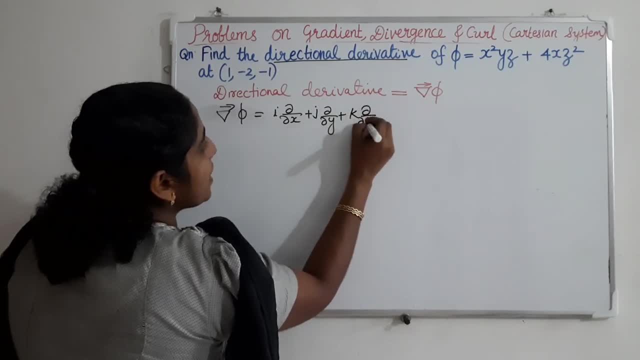 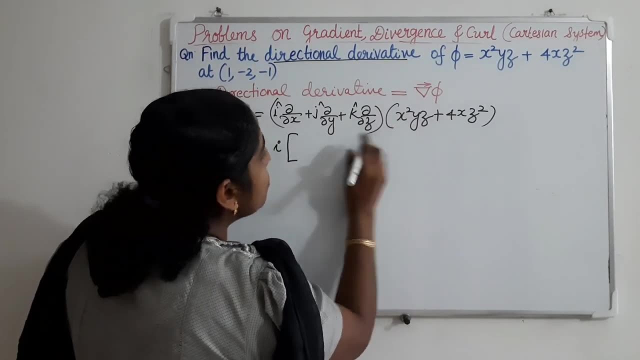 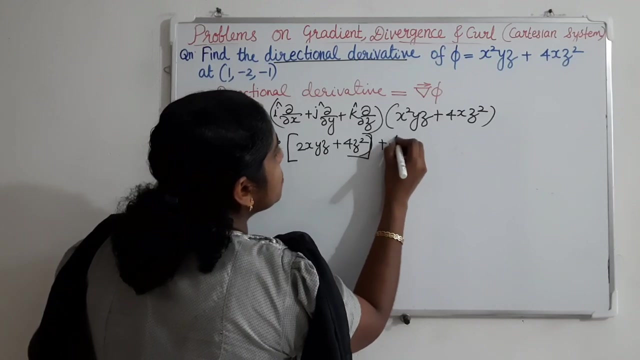 dou y plus k, dou by dou z, which operate on the scalar function That is equal to i, into dou by dou x of this, That is, 2xyz plus 4z, square plus j, into dou by dou y of partial derivative of this function. 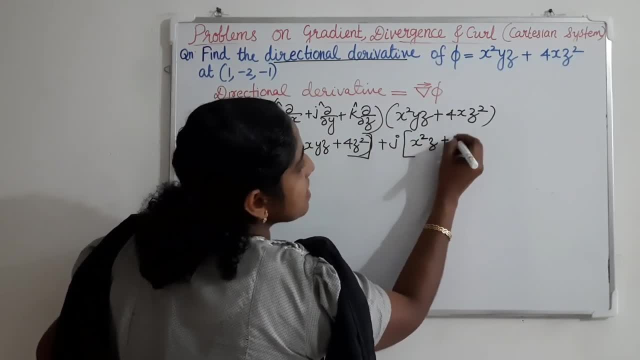 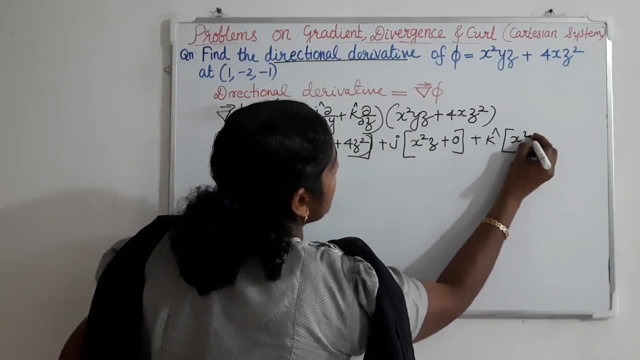 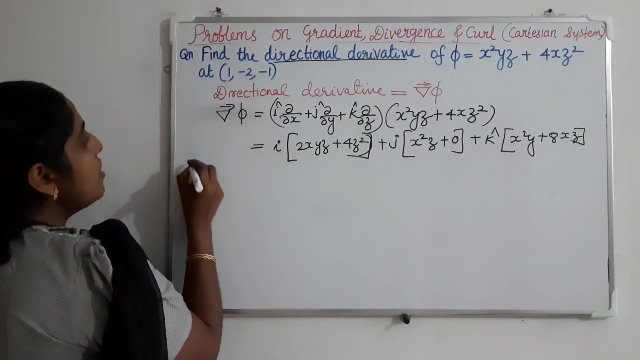 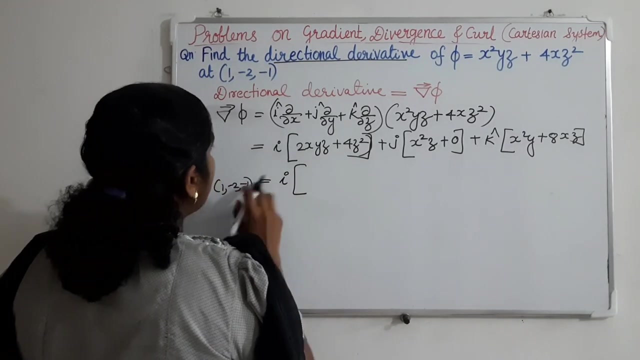 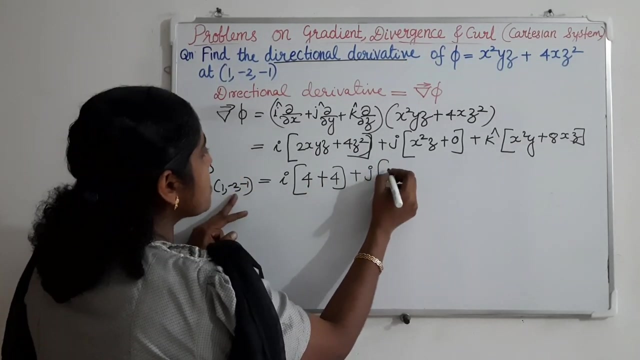 Now we have to find out this: del phi at 1 minus 2 minus 1, point, That is equal to i, into 2, into xyz, That is 4 plus 4z square, that is 4.. Now we have to find out this: del phi at 1 minus 2 plus j, into x square z, that is minus 1 plus k, into x. 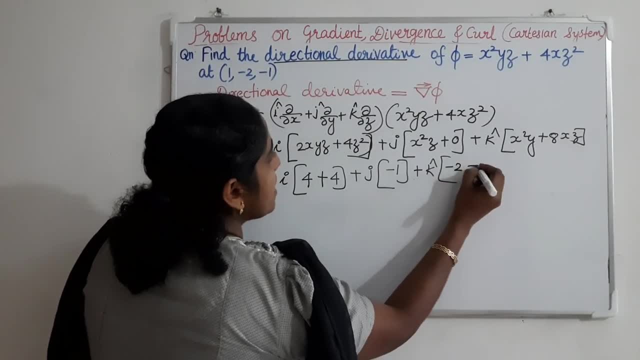 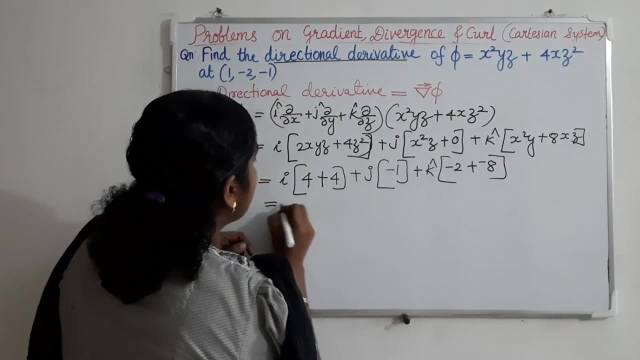 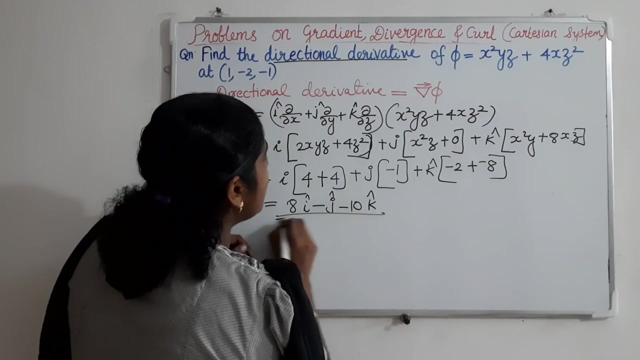 square y, that is minus 2 plus 8, into xz, xz is minus 1, into 8 is minus 8.. So that is equal to 8i minus j minus 10k. So this is the directional derivative of the given function. 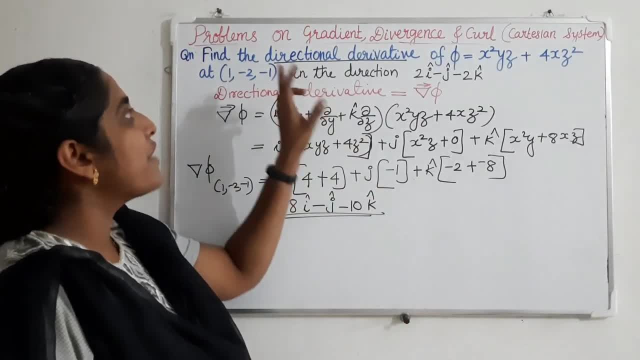 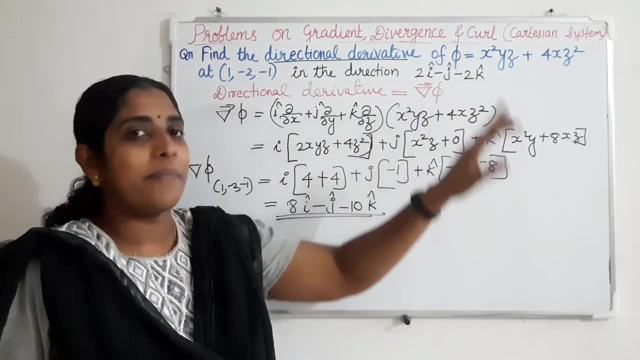 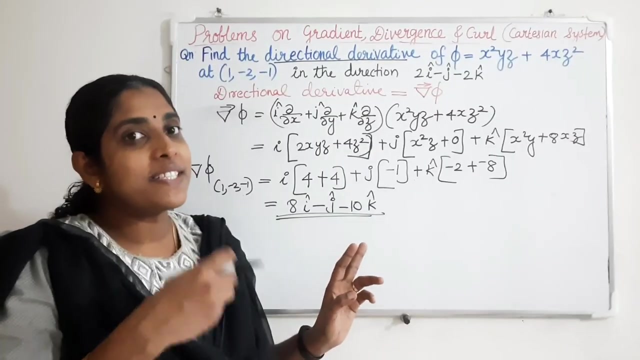 Now, in the same question, there is some modifications. Find the directional derivative of this function at the given point, in the direction 2y minus j minus 2k. We have found the directional derivative at 1 minus 2 minus 1.. So in order to find out this, 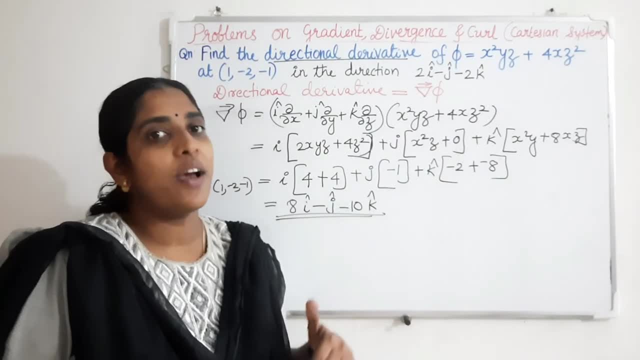 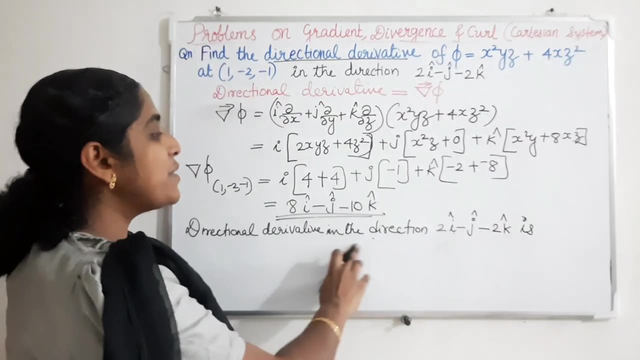 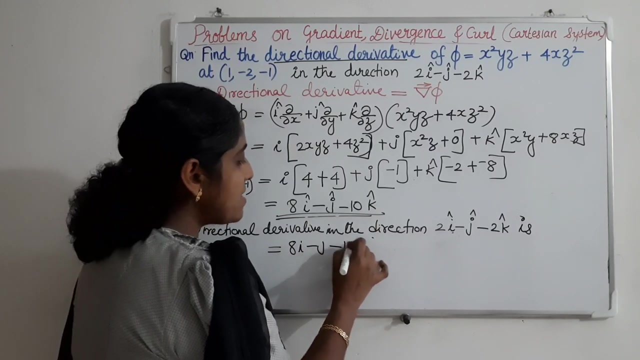 directional derivative in a particular direction. what we have to do, we have to just multiply it with the unit vector along that direction. Therefore, directional derivative in the direction 2y minus j minus 2k is del phi, that is 8.. So 2i minus j minus 10k dot unit vector along this direction. What will be the unit vector? 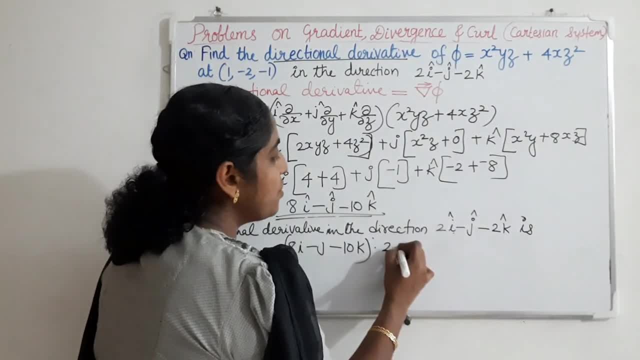 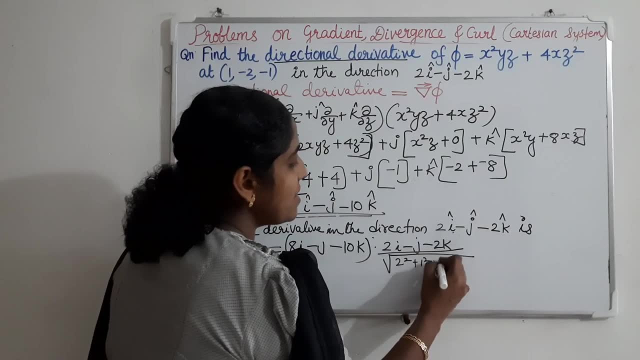 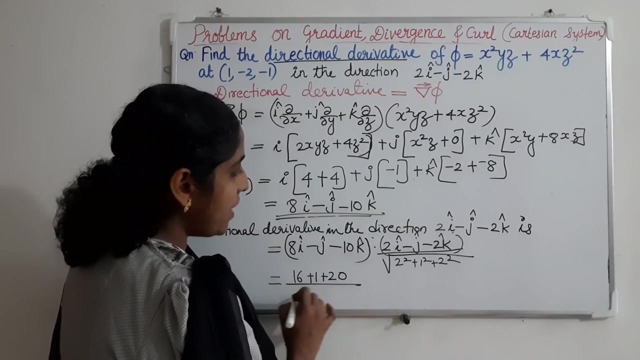 This vector divided by its magnitude, that is, 2i minus j minus 2k, divided by square root of 2 square plus 1 square plus 2 square, That is equal to 16 plus 1 plus 20. divided by root of 4 plus 4, 8 plus 1, 9.. So that is equal to 2i minus j minus 10k. Personalization of the denominator unit vector. along this direction, Simplified Discussion is completed. What we have to do In the same question, however, let's find out its elements. Is there something which has changed? 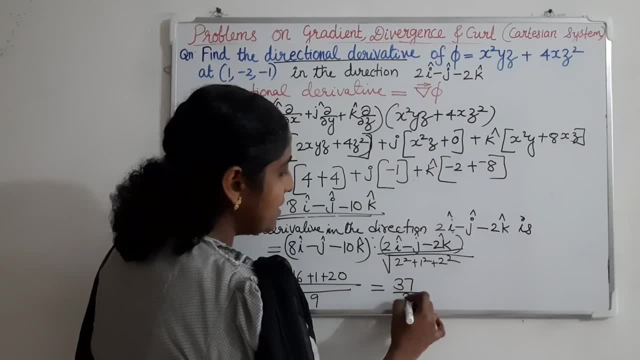 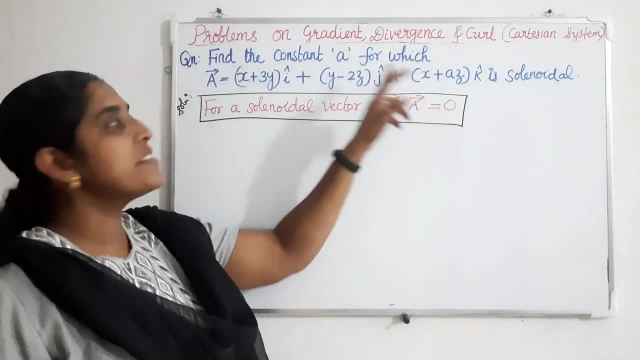 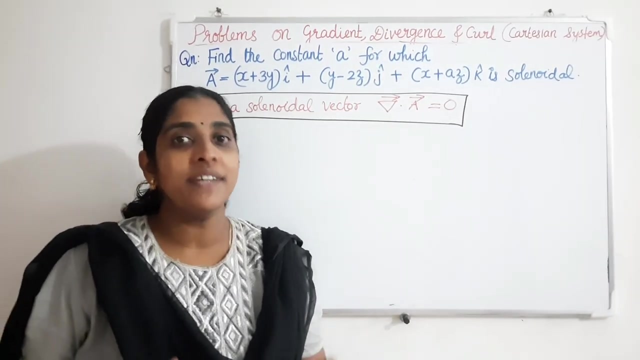 to 37 divided by 3.. So this is the directional derivative in the given direction. See the next question. Find the constant A for which the given A vector is solenoidal. What is the meaning of solenoidal? If the divergence of a vector function is 0, that vector function is solenoidal, That is. 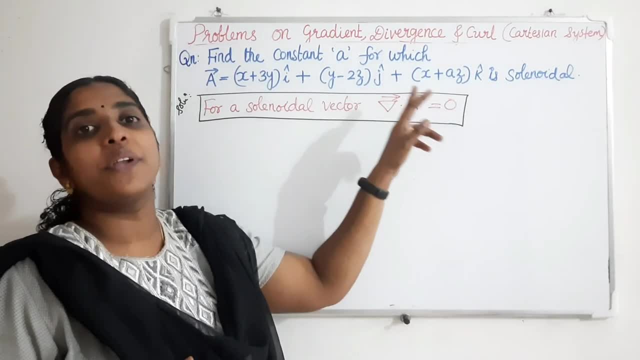 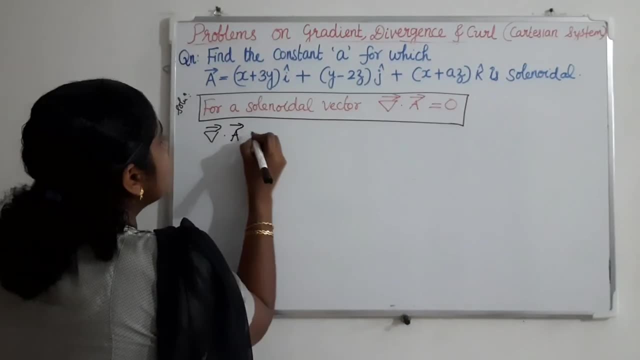 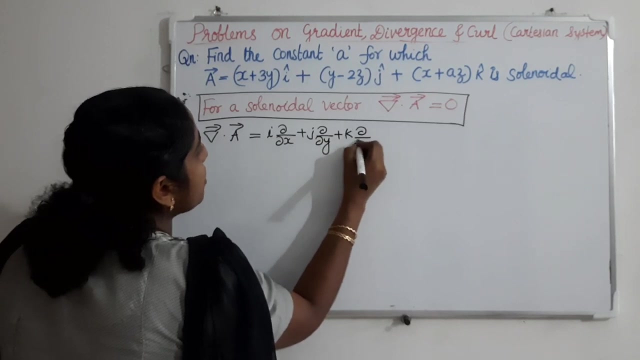 for a vector A to be solenoidal, del dot A must be 0.. So we can apply this concept here. So what is del dot A here? That is I, dou by dou x plus j, dou by dou y plus k, dou by dou z dot A. 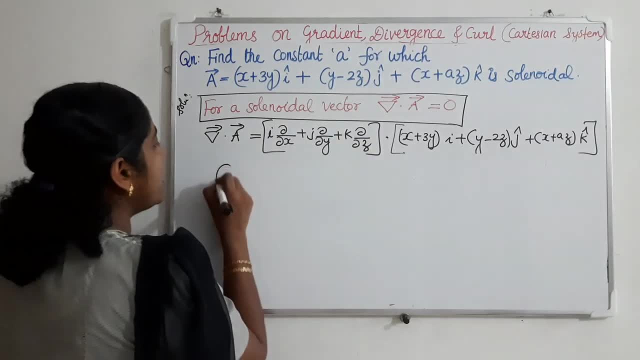 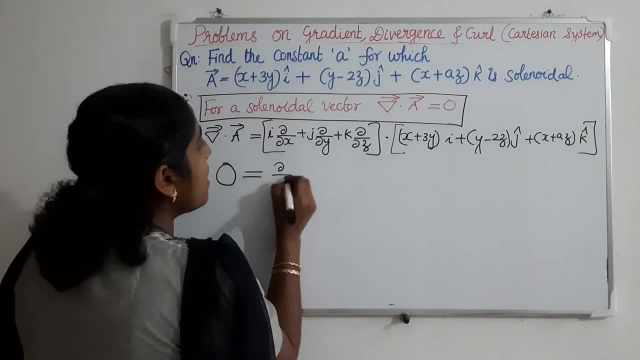 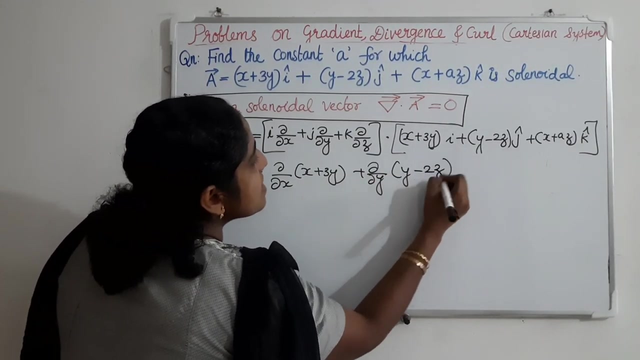 vector. For solenoidal vector, this del dot A is equal to 0. That is equal to dou by dou x of x plus 3y Plus dou by dou y of y minus 2z plus dou by dou z of x plus Az. Dou by dou x of x plus 3y is 1.. 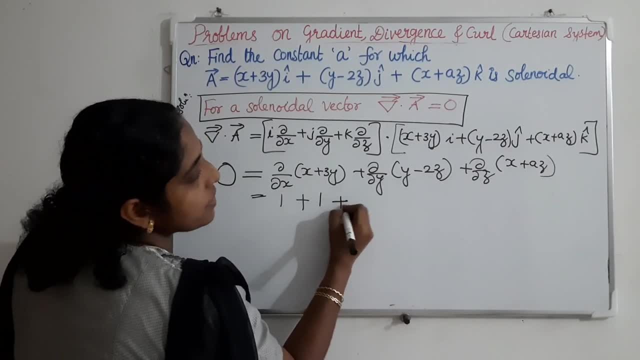 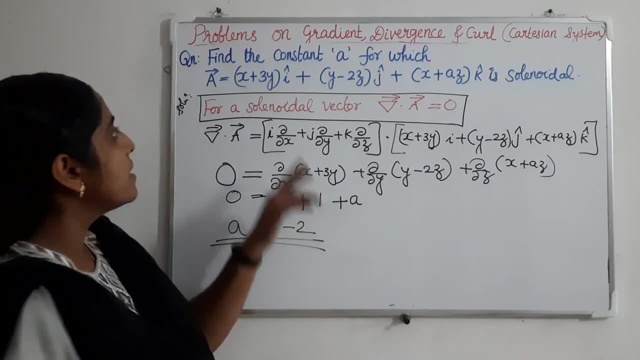 Dou by dou y of y minus 2z is 1.. Dou by dou z of x plus Az is A. That is, A is equal to minus 2.. So for a vector, this, to be solenoidal, the constant A value is minus 2.. 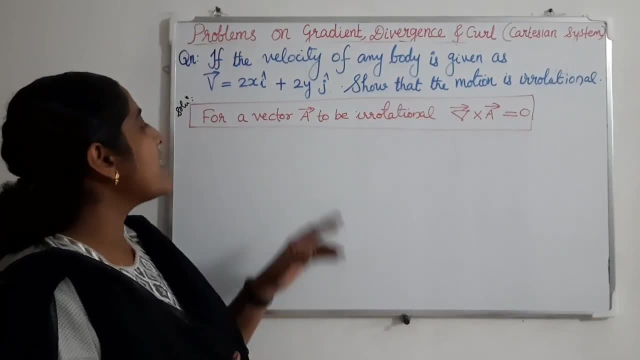 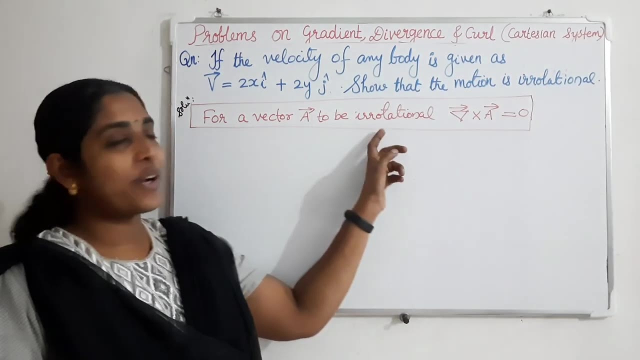 See the next question. If the velocity of any body is given as V vector equal to 2xi plus 2yj, show that the motion is irrotational. For a vector to be irrotational, that curl of that vector must. 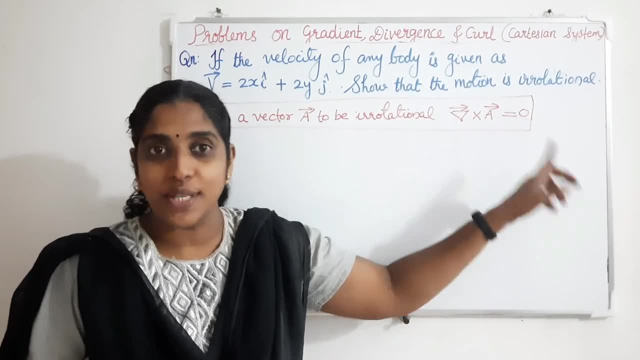 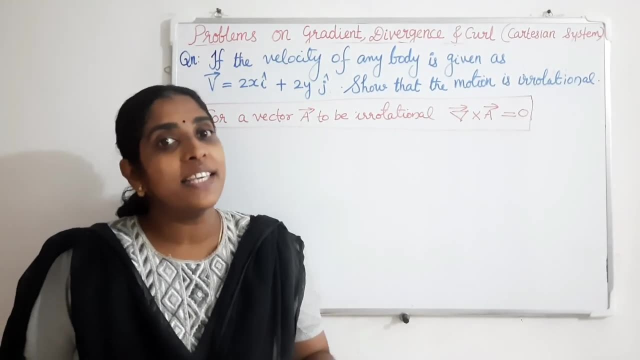 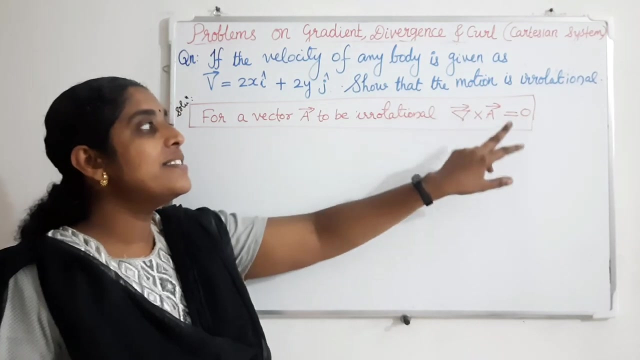 be 0. That is del cross A is equal to 0. Then we can say that A vector is irrotational. That is physical significance of curl. Curl gives how much the given vector is rotating around the given point. So if the curl is 0, that means that vector is irrotational. So we can find out the curl of the. 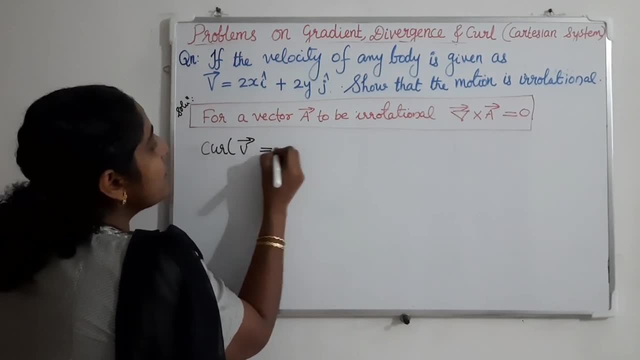 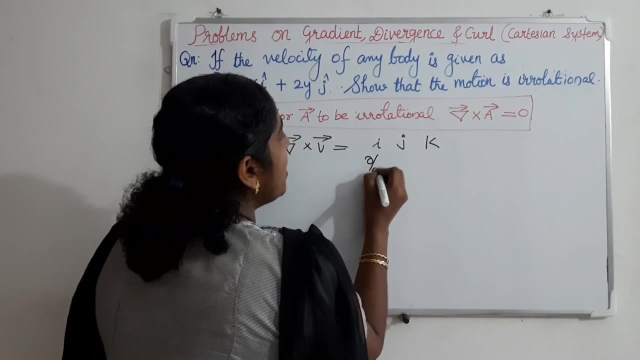 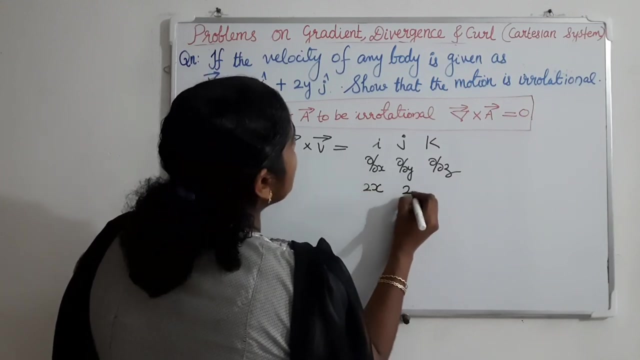 given velocity, That is curl. V is equal to del cross, V is equal to ijk dou by dou x, dou by dou y, dou by dou z. V vector is 2xi 2yj. There is no z component, So here it is 0.. That is i into. 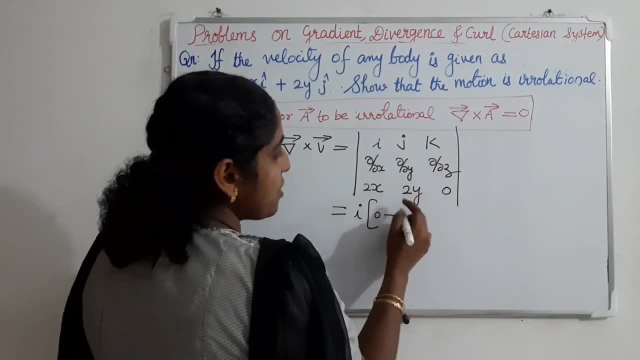 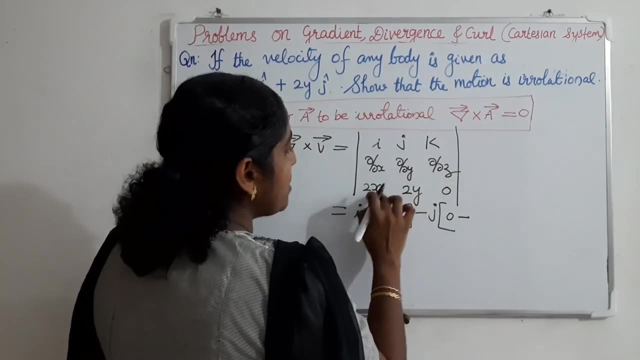 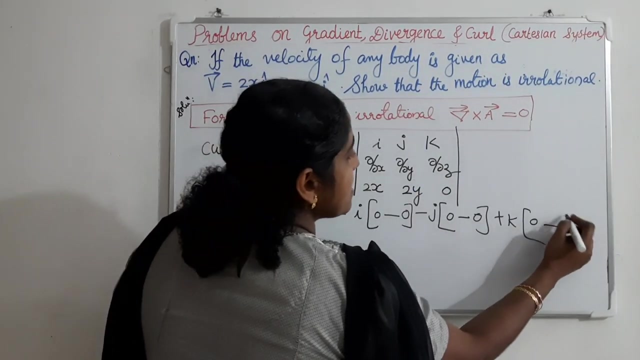 dou by dou y of 0 is 0, minus dou by dou z of 2y, That is also 0 minus j. into dou by dou x of 0 is 0, minus dou by dou z of 2x is 0 plus k. into dou by dou x of 2y is 0 and dou by dou y of 2x is 0. 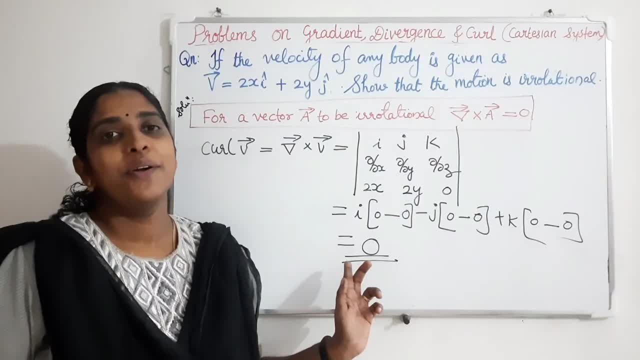 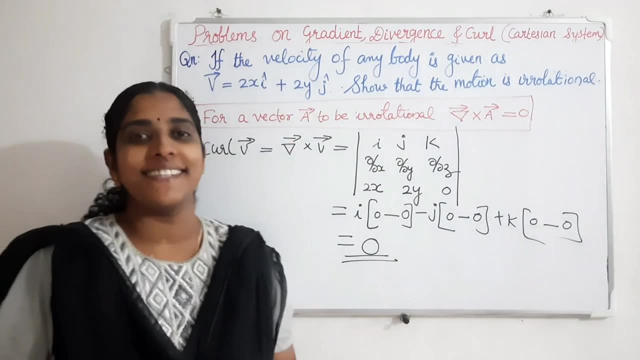 That means we are getting a 0 vector. Due to this 0 curl, we can say that the motion which is described by the given velocity vector is irrotational. This is the next question. The electric potential in a region of space is given by V equal to. 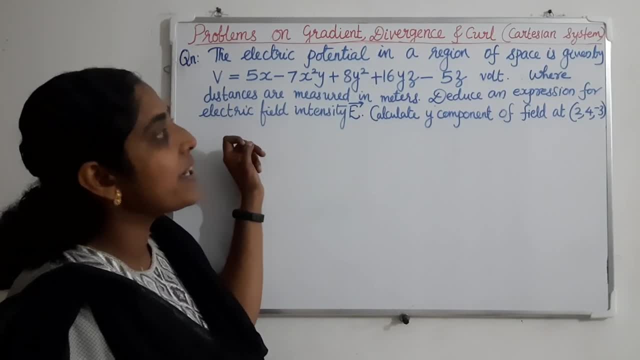 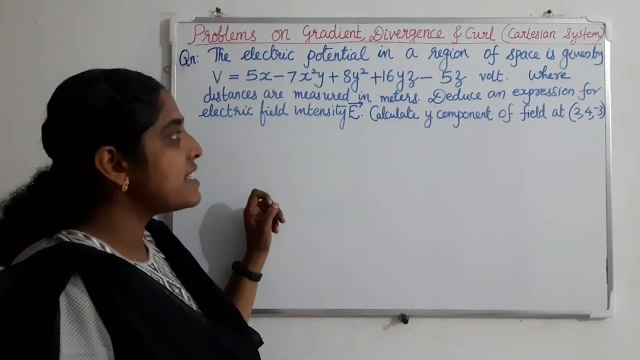 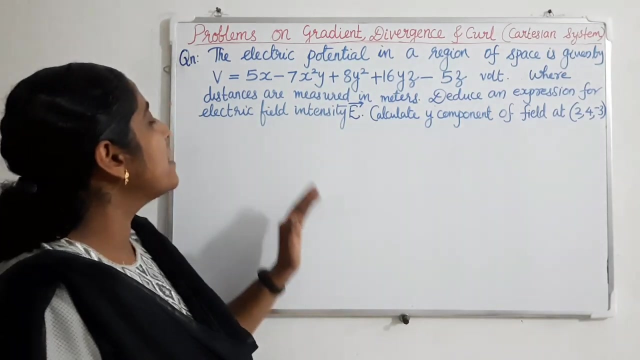 5x minus 7x square y plus 8y square plus 16yz minus 5z volt, where distances are measured in meters. Reduce an expression for electric field intensity, E vector. Calculate y component of the field at 2, 4, minus 3.. That is in this question. the potential function is given From that. 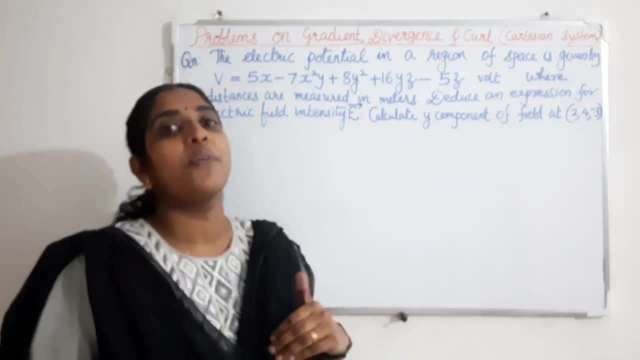 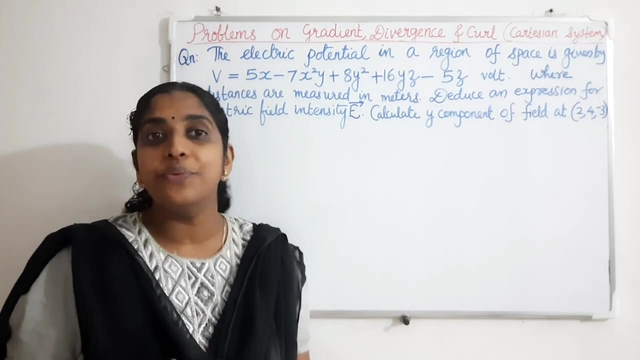 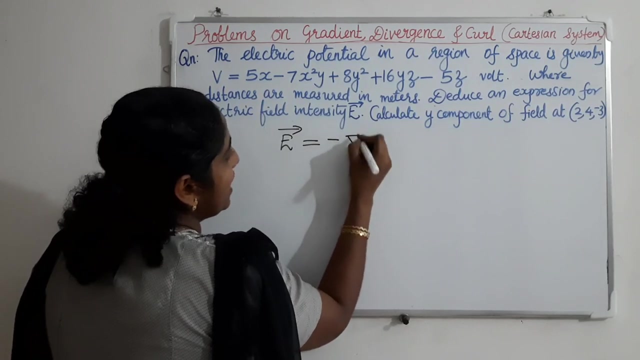 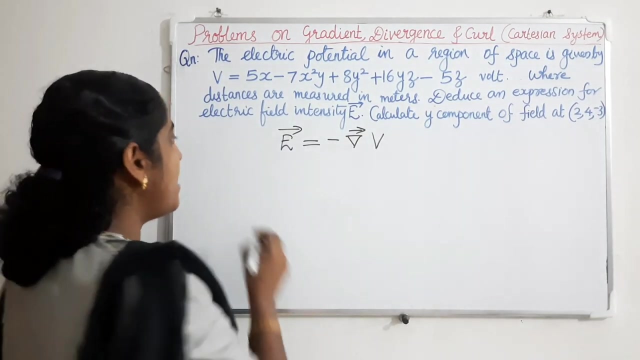 potential function. we have to find out the expression for electric field intensity, How this electric field is related to the potential. Electric field is the negative gradient of potential function, That is, E is equal to minus del V. When this del operate on the scalar potential function we will get the electric field That is. E vector is: 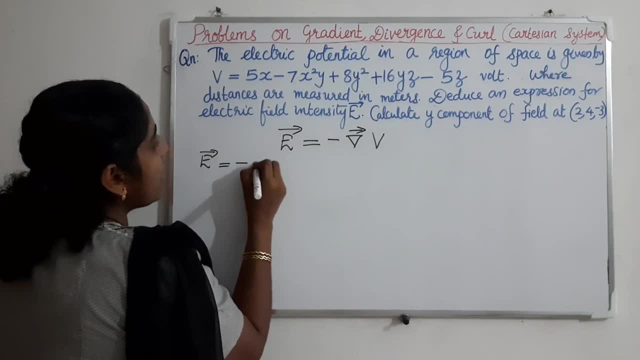 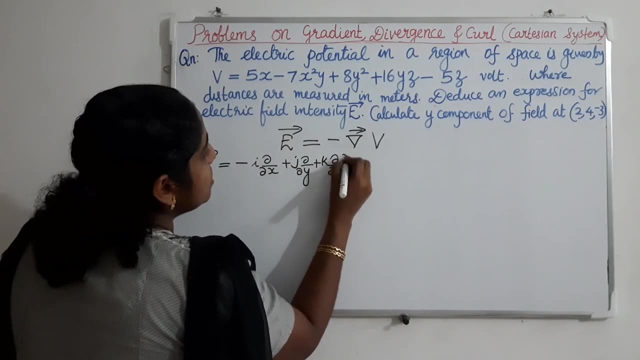 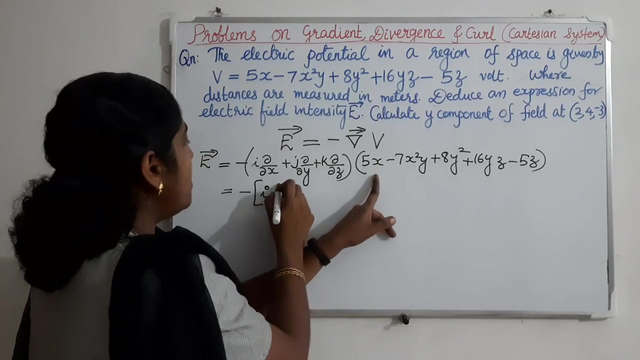 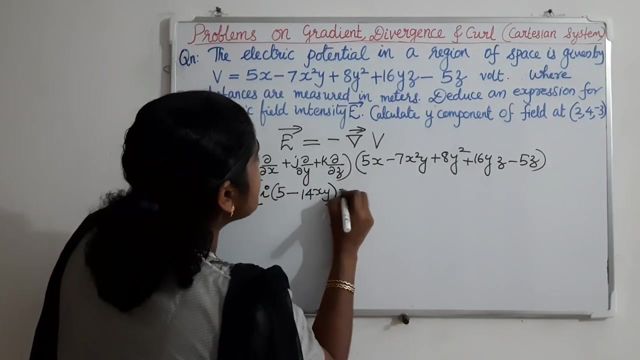 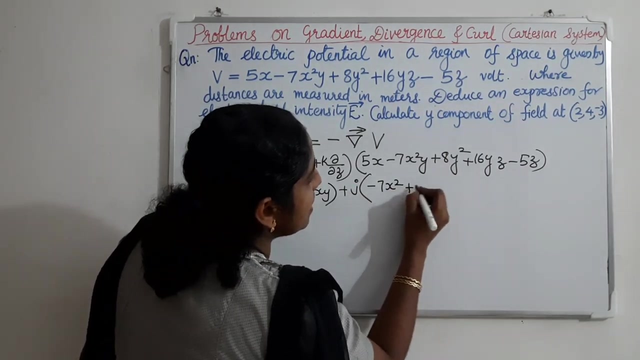 equal to minus del vector is i. dou by dou x plus j. dou by dou y plus k. dou by dou z into V, That is minus i. into dou by dou x of this function, That is 5 minus 14xy plus j into dou by dou y of this function is minus 7x square Here. y term is there, That is 16y. 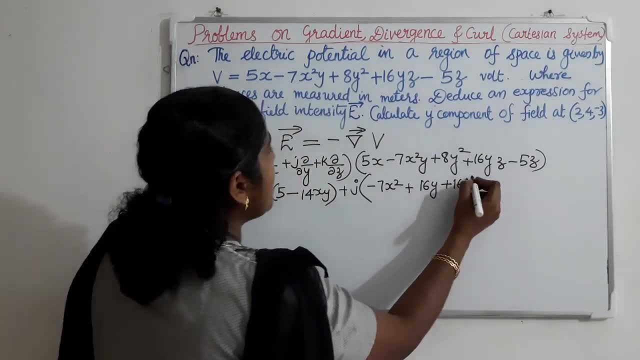 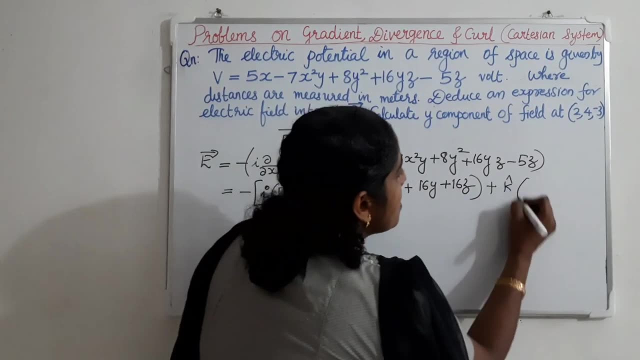 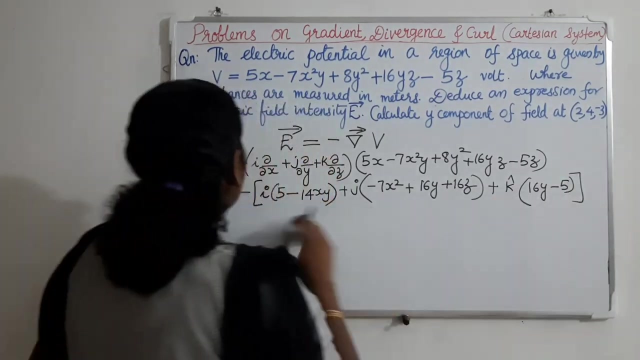 plus here 16z plus k. into dou by dou z of this function, z components are 16yz derivative is 16y minus 5.. So this is the expression for the electric field intensity from the potential function. Here the distances are: 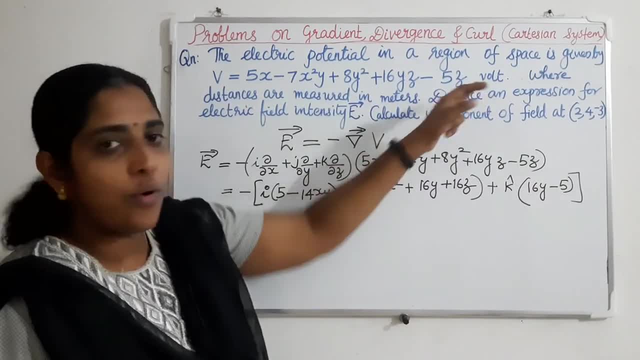 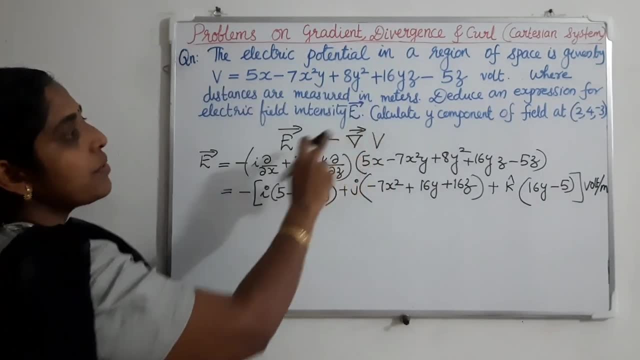 measured in meters. The potential is given in volt, So the unit of electric field will be volt per meter. So now we have to find out the y component of the electric field intensity. So what is the y component of this field? at 2,, 4, minus 3? What will be the y component from this? 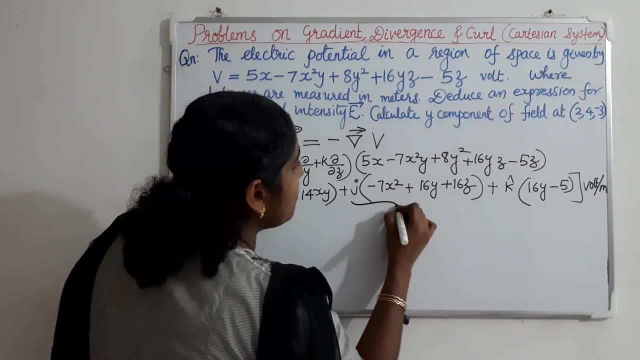 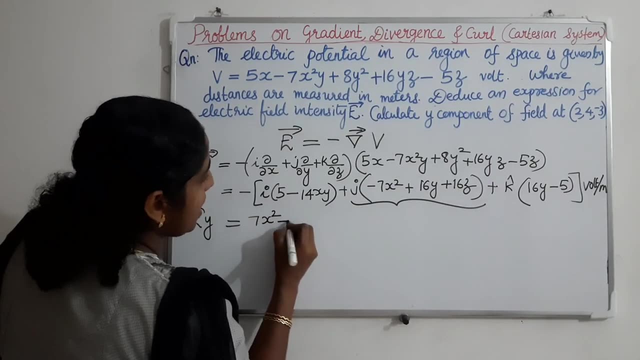 expression. Y component means the component of j, So minus is outside. That is minus of this component. That is 7x square minus 16y minus 16z. Now what is the y component at the 2,, 4,? 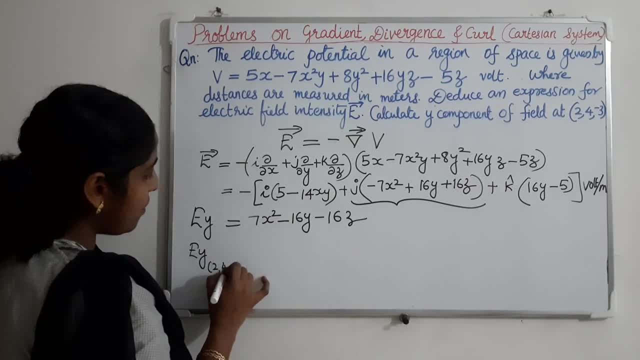 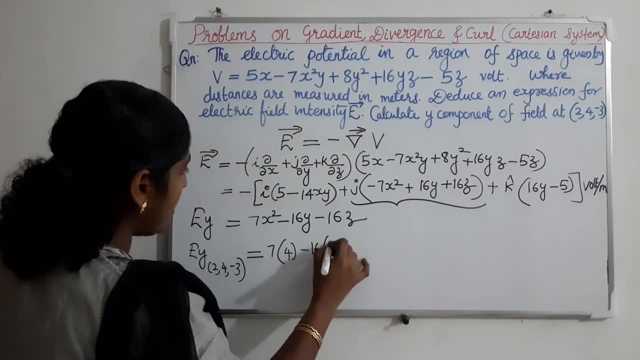 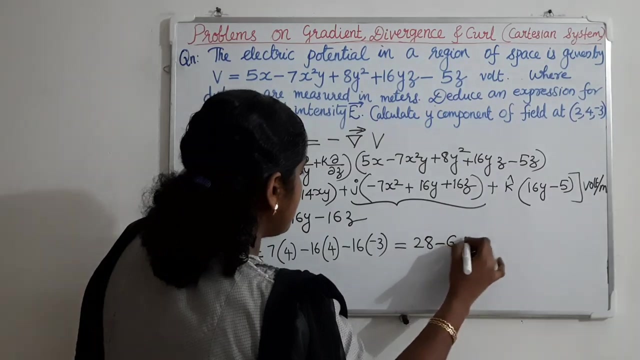 minus 3. point. Therefore E, y, 2, 4, minus 3 is equal to 7 into 2, square is 4 minus 16. into y is 4 minus 16, into z is minus 3.. That is 28 minus 64 plus 48.. That is. 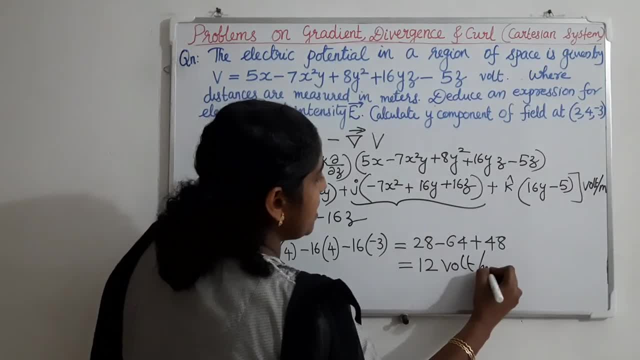 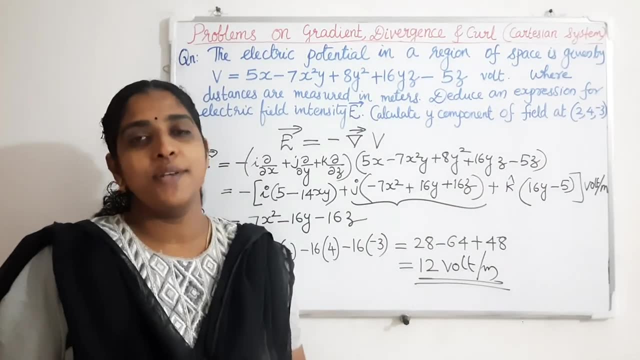 equal to 12 volt per meter. So the y component of the electric field at the 2,, 4, minus 3 is 12 volt per meter. So if the potential function is given, from the potential value we can find out the. 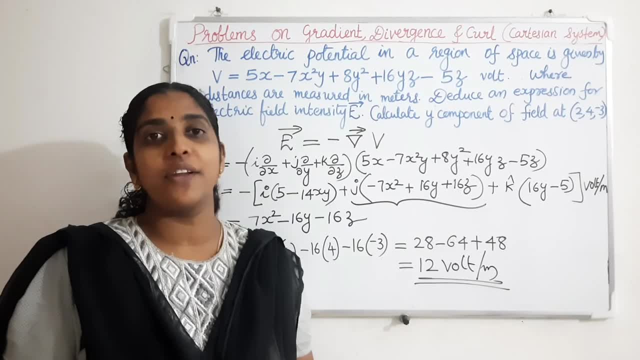 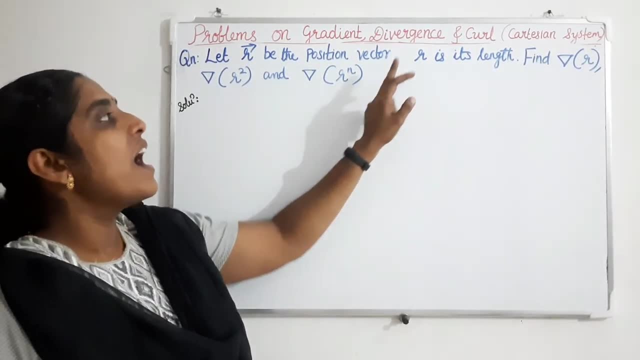 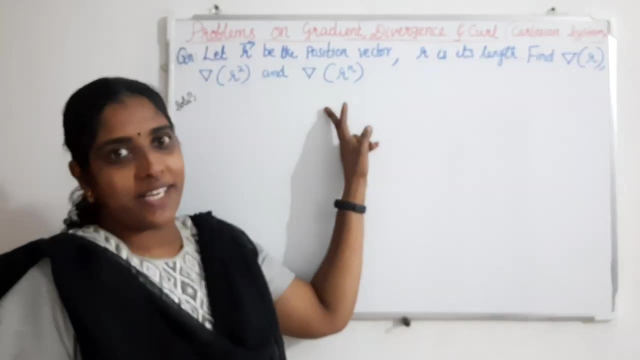 electric field as the negative gradient. So we can find out the electric field as the negative gradient of potential. Here we are using the concept of gradients. See the next question. Let r vector be the position. vector r is its length. Find del of r, del r, square del r raised to n. So in this, 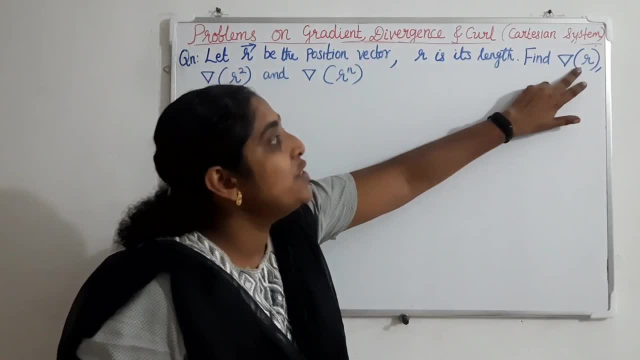 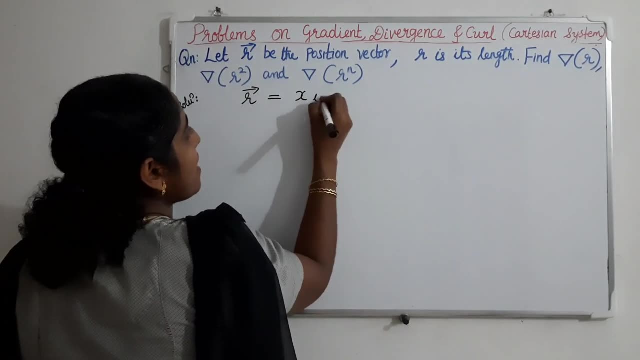 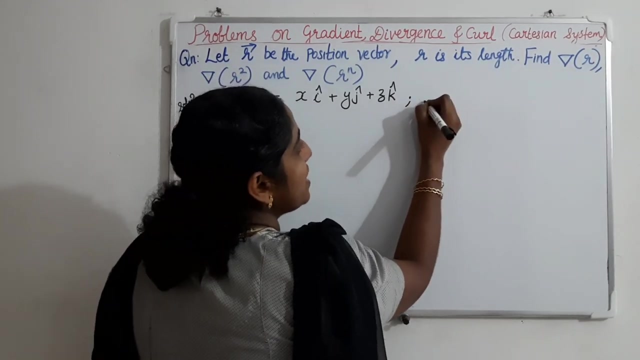 question. we have to find out the gradient of the magnitude of the given vector. So what is a position vector? Position vector we can represent in Cartesian coordinates as xi plus yj plus zk. Then what will be its magnitude, its length? That is modulus of r vector That is equal to root. 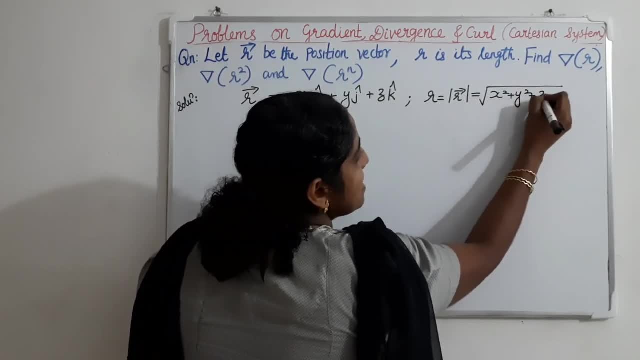 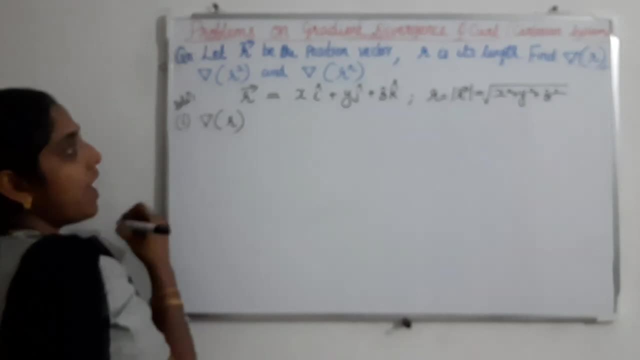 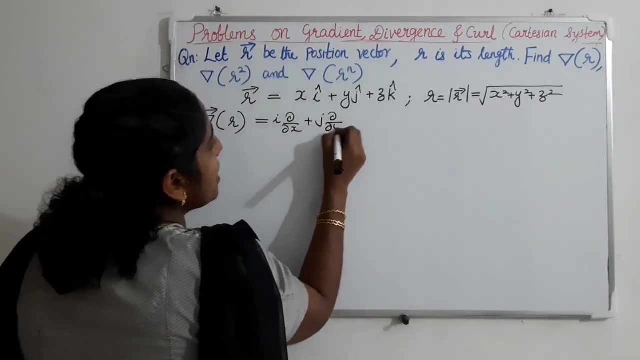 of x square plus y square plus z square. So first we have to find out the del of this magnitude of this vector del r, That is equal to i dou by dou x plus j, dou by dou y plus k dou by dou z into. 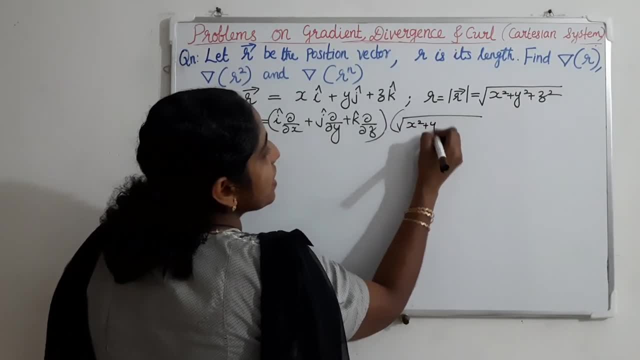 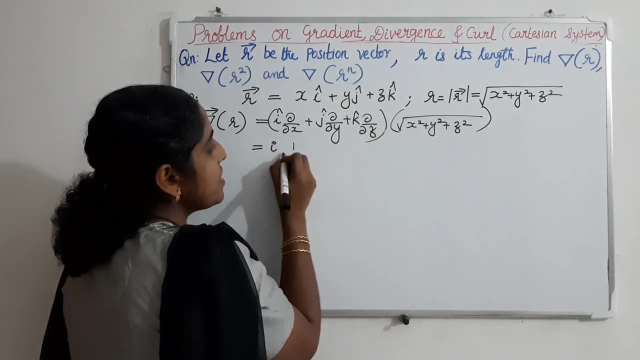 r, r is root of x square plus y square plus z square, So that is equal to i into dou by dou. x of root of this function is 1 by 2, root of x square plus y square plus z square into derivative of. 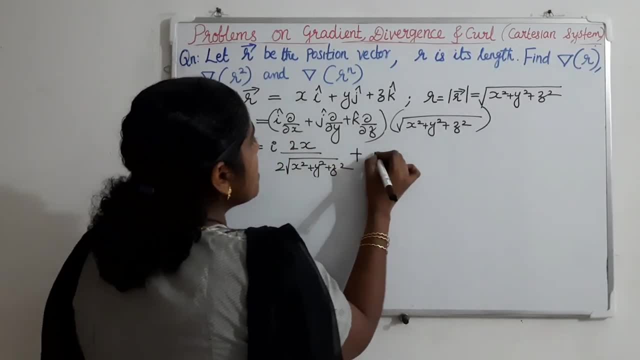 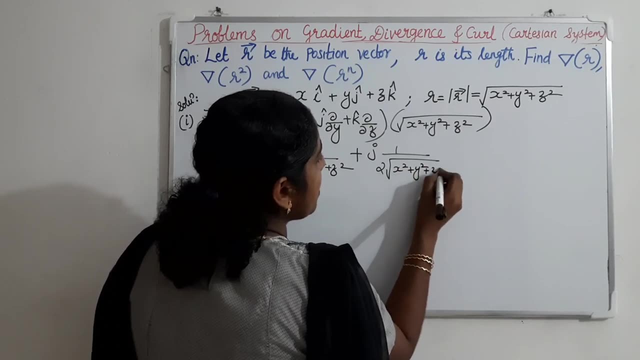 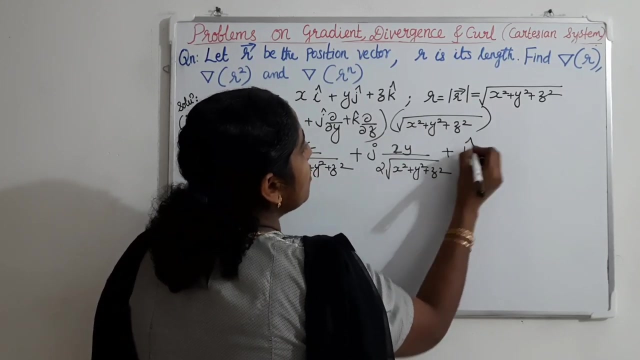 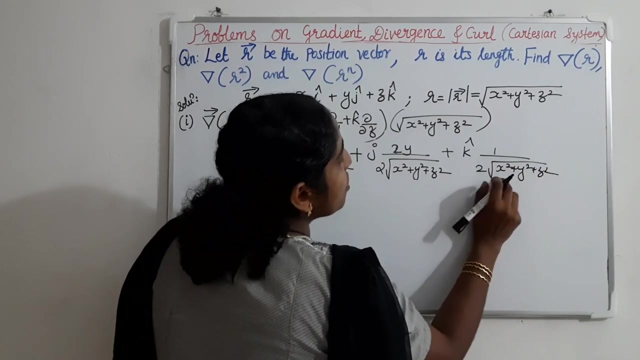 this function, that is 2x plus j, into dou by dou. y of this function is 1 by 2. root of x square plus y square plus z, square into. partial derivative of this function with respect to y, that is 2y plus k into dou by dou. z of this function is 1 by 2 root of x square plus y square plus z, square into. 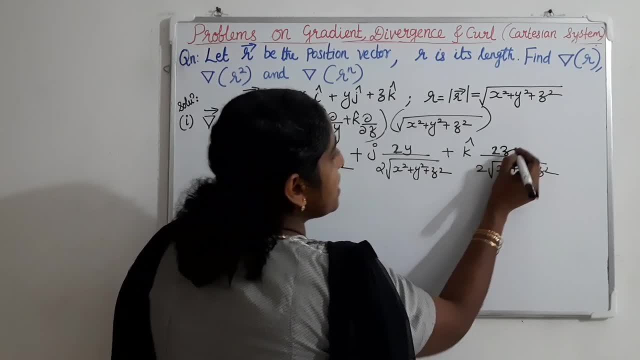 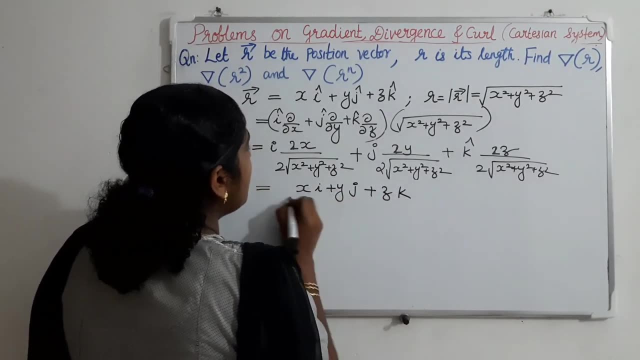 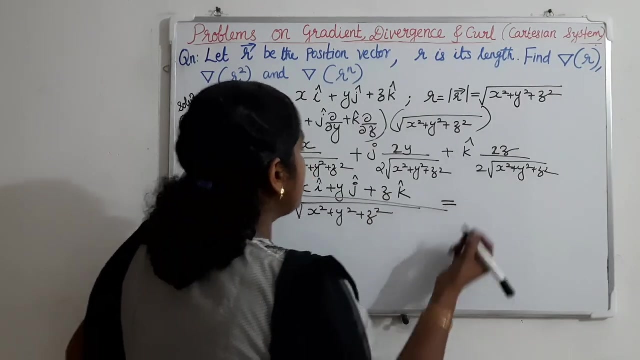 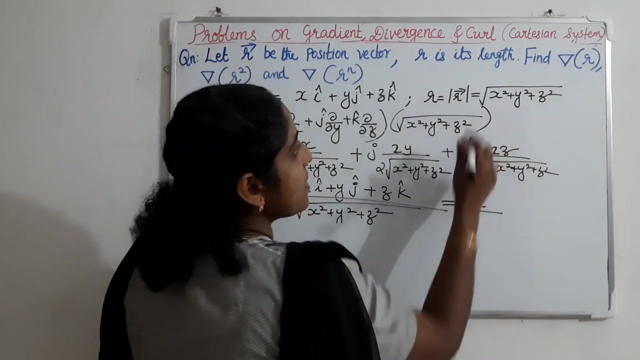 partial derivative of this function. with respect to z, that is 2z, We will get it as xi plus yj plus z square plus z square. That is equal to xi plus yj plus zk. is r vector divided by root of x square plus y square plus z is modulus of r vector. So r vector divided by modulus of r vector is r. 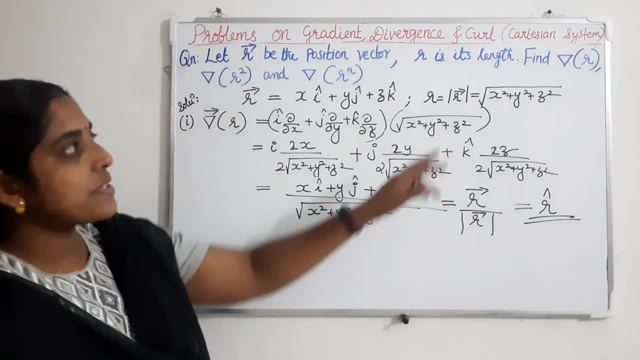 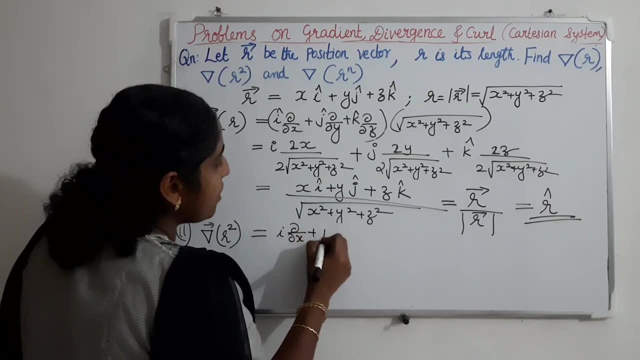 capital is the unit vector. The next question: we have to find out the del of r square That is equal to i dou by dou x plus j dou by dou y plus k dou by dou z. Next, we have to find out the del of x square plus y square plus z square into r square is x square. 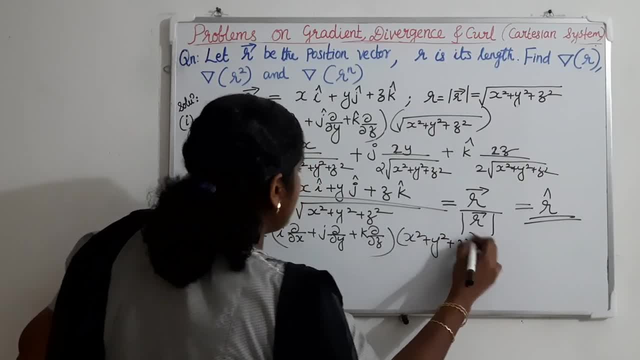 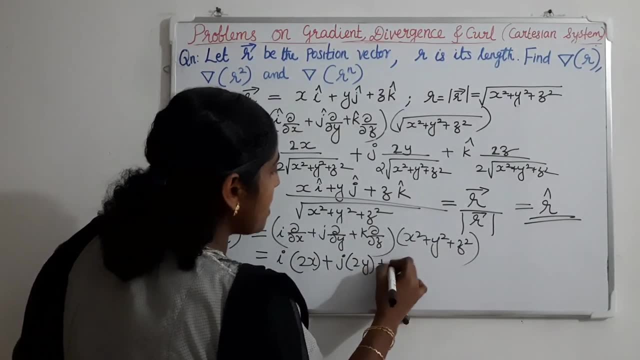 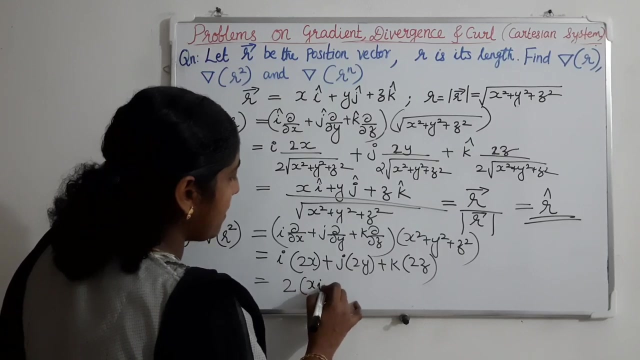 plus y square plus z square, So that is equal to i into dou by dou, x of this is 2x plus j into 2y plus k into 2z, That is, 2 into xi plus yj plus zk. What is this? xi plus yj plus zk, That is r. 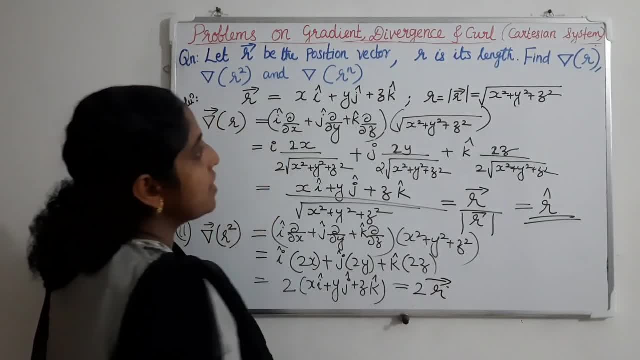 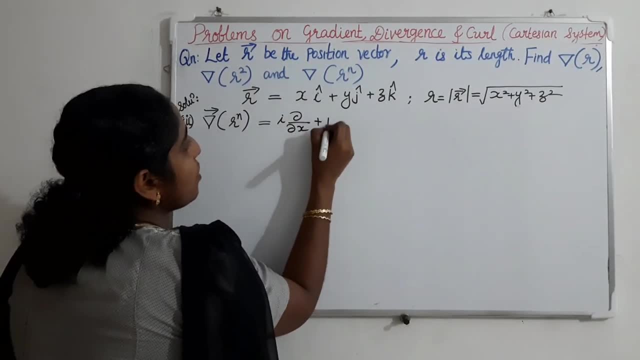 vector. So the answer is 2r vector. Next we have to find out the del of x square plus yj plus zk. That is, i dou by dou x plus j, dou by dou y plus k, dou by dou z into r raised to n. So in general, 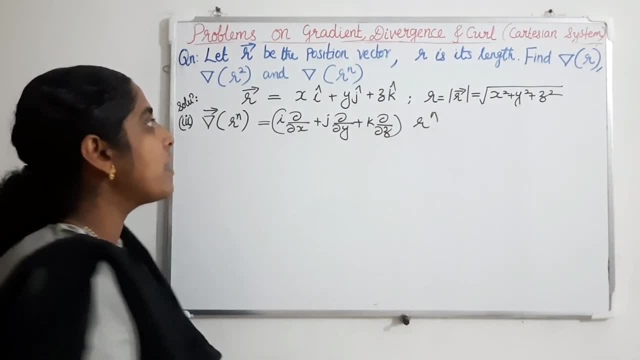 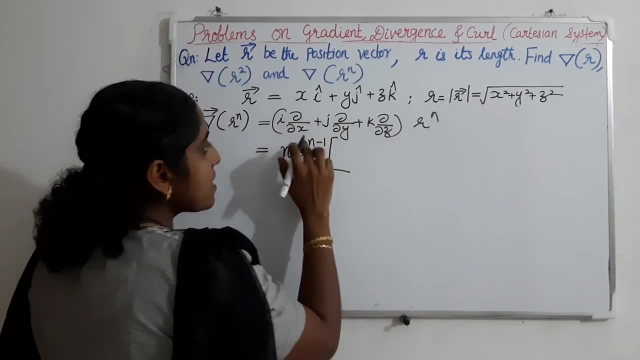 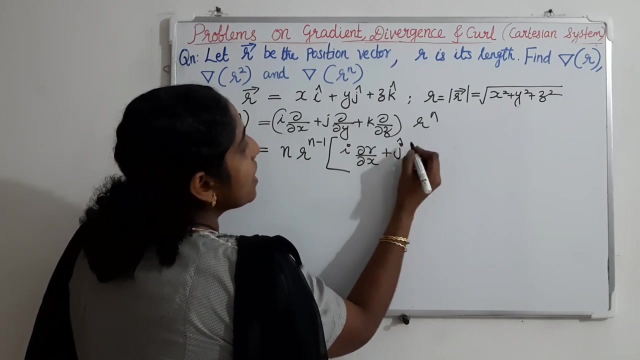 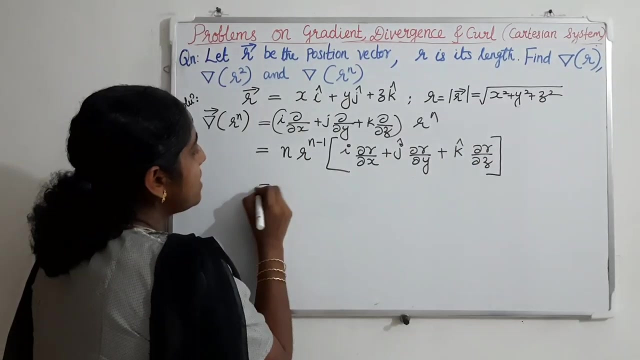 if we are taking the nth power of r, the differential will be n? r raised to n minus 1 into this x component derivative will be i dou r by dou x, plus y component will be j dou r by dou y and this component will be k dou r by dou z. That is equal to n r raised to n minus 1..